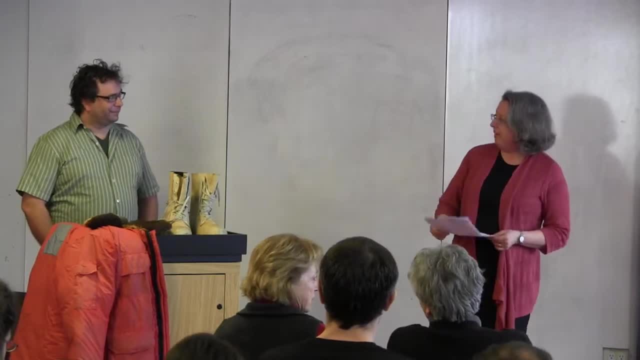 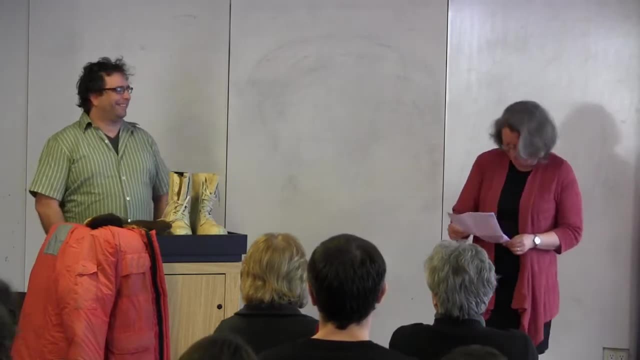 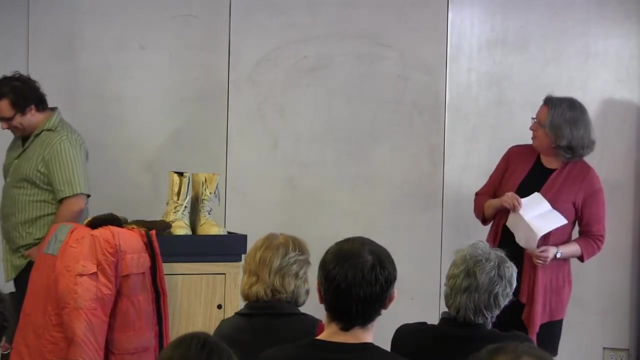 level change. And just two interesting facts about Mike. He's been to Antarctica 12 times and the Arctic twice. He's a very hardy soul And in 2008, the US Board of Geographic names named a ridge after him, and it's actually called Lewis Ridge. So can you find it on Google. 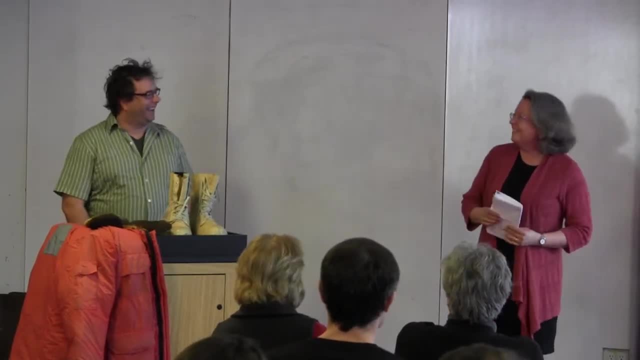 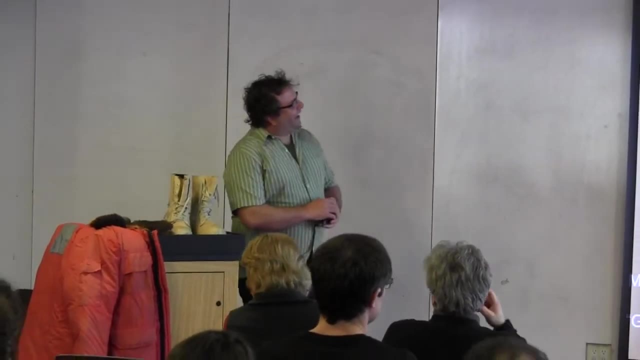 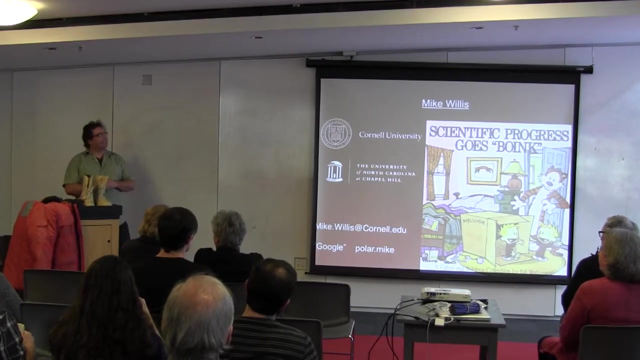 Maps. You can find it on Google Maps. So welcome Mike. Thank you, Rose. So thank you for having me. I'd like to show some work entitled Scientific Progress. Goes Point, Bill Walterson with Calvin on the topic of scientific progress, And I'm going to give you a little bit of background on the research that I'm working on. So I'm going to show you some of the research that I'm working on. I'm going to show you a little bit of the research that I'm working on And I'm going to show you a little bit of the 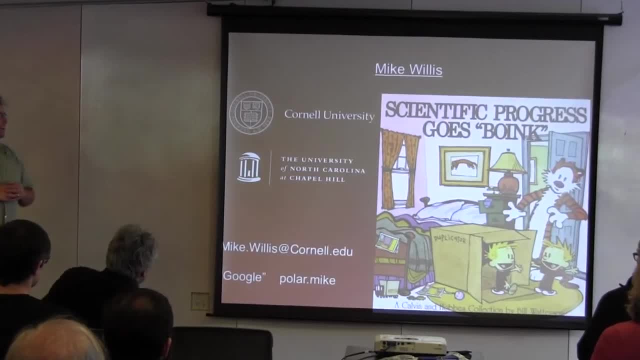 things that I'm working on And unfortunately it's hard for hardworking people if we don't know that science works and legally And if people understand the science we can get the right results. But there would be lots of research that you can do that I can stick to. I've worked with 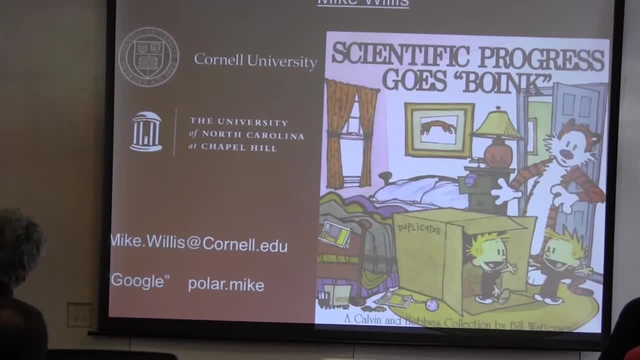 many experiments in. Paulo Logs did a lovely gentle representation of science through these cartoons. You can get these cartoons. There's lots of good stuff about how science should work, doesn't work, does work and what society thinks of it. So I thought it was an appropriate playful. 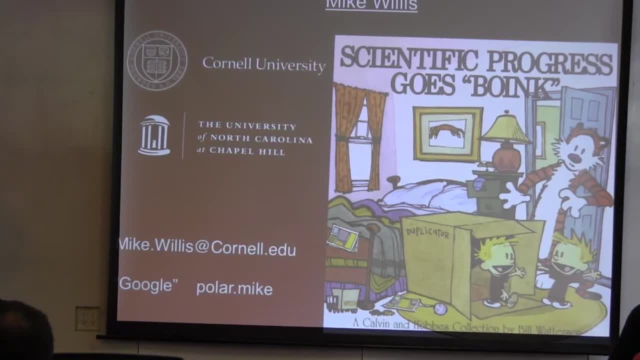 to look at how Earth goes boink when you load it with the mass or take a mass away. So, if you're interested, during my times in Antarctica and Greenland I took quite a lot of photos. If you Google Polar dot Mike, you'll find Lot's of photos showing this alien. 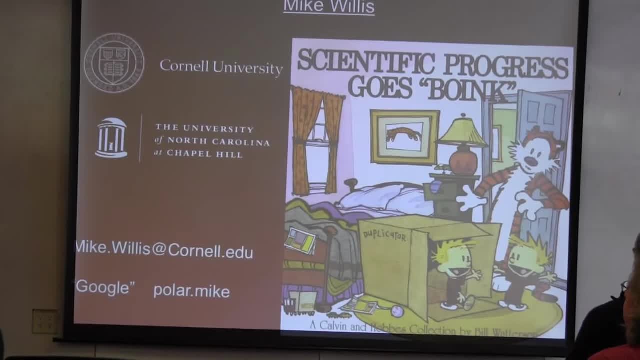 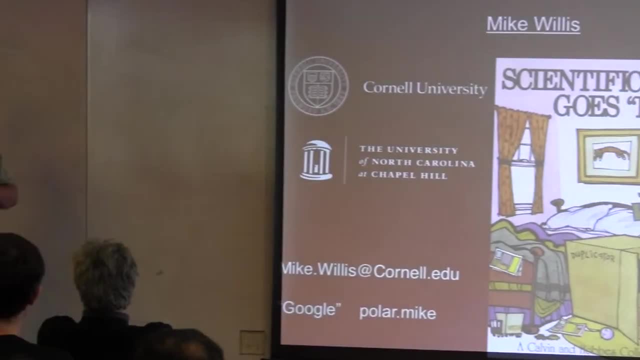 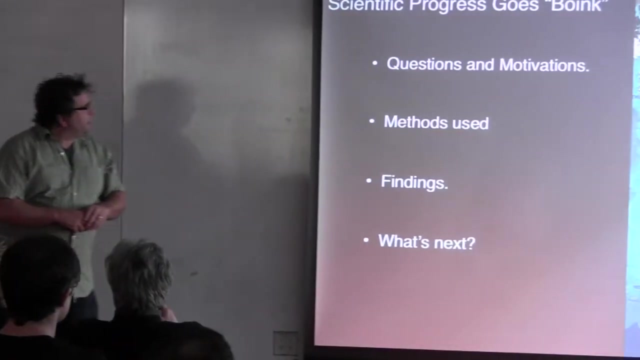 You'll find a lot of my photos online, when the first hit genuinely comes from Google, And if you ever use Google Earth and look around and click on photos and then you'll find a lot of them that I take about myself. So scientific progress goes boink. 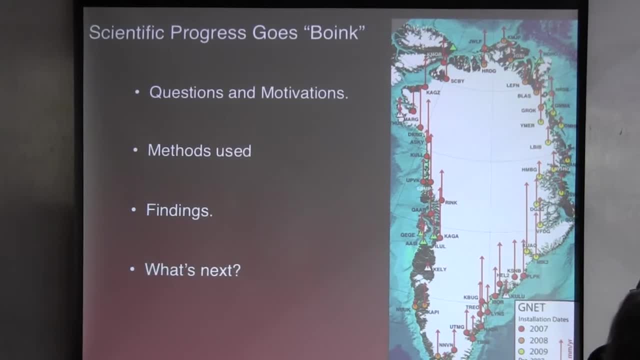 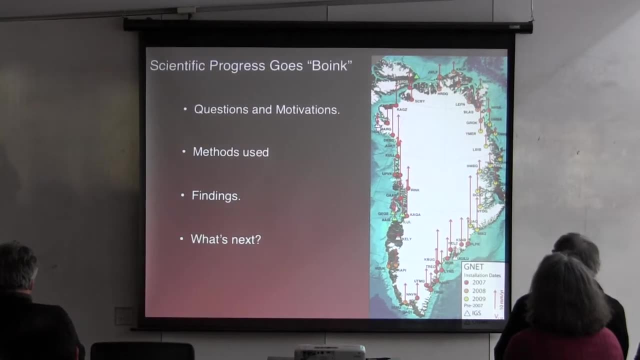 I'm going to talk about some of the questions and motivations, why I'm looking at what I'm looking at, The methods used, the findings and what next. And I'm going to concentrate mostly on Greenland, just because, well, to be blunt, Greenland's- 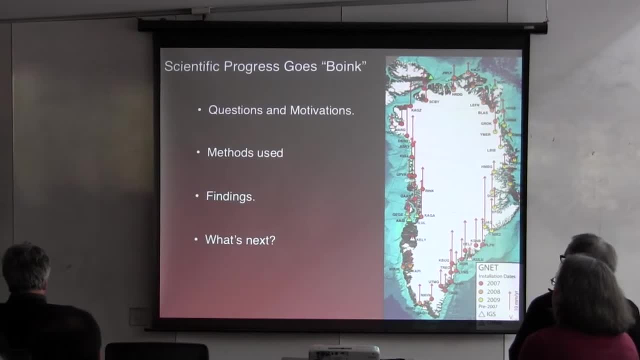 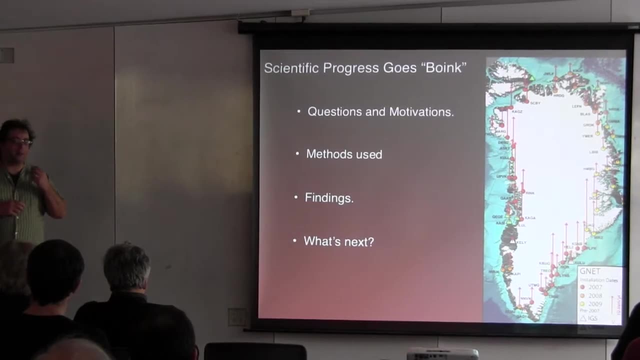 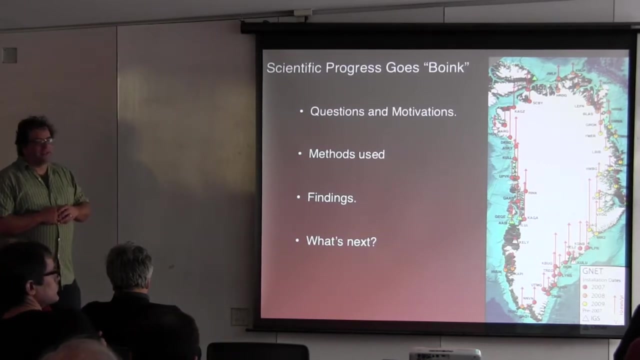 easier. Antarctica is still a very complicated problem. The problems in Antarctica are due to the ice. they're changing just now and having a big long-term memory, So I'll cover what that means a little bit later. Whereas Greenland itself is, the singles are so large. 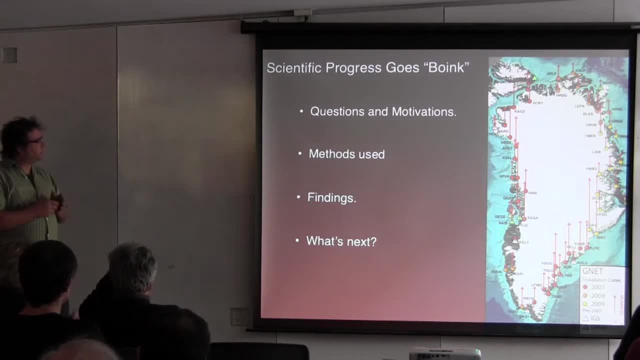 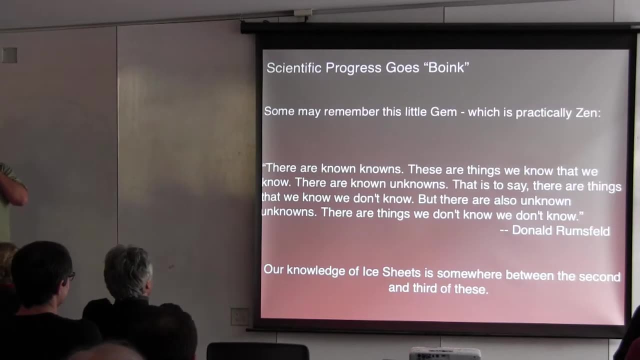 What we measure is so large that it's pretty compelling. It's an easier story. Some of you might remember this little gem from Donald Rumsfeld, which I feel is practically zen: There are known, knowns. These are things that we know, that we know. 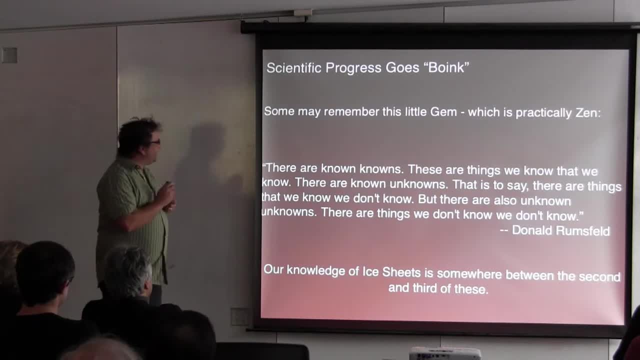 There are known unknowns, That is to say, these are things that we know, that we don't know, But there are also unknown unknowns. These are things that we don't know, that we don't know, And I like to break this down. 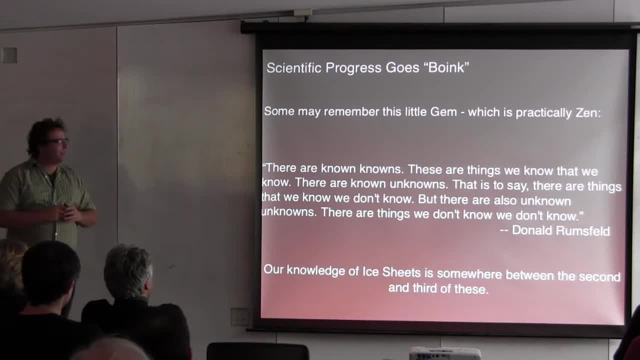 Known knowns, I'm going to call them facts. I could have said: there are facts, Then there are known unknowns. I'm going to call those questions. And then there are things we don't know. we don't know, I'm going to call them surprises. 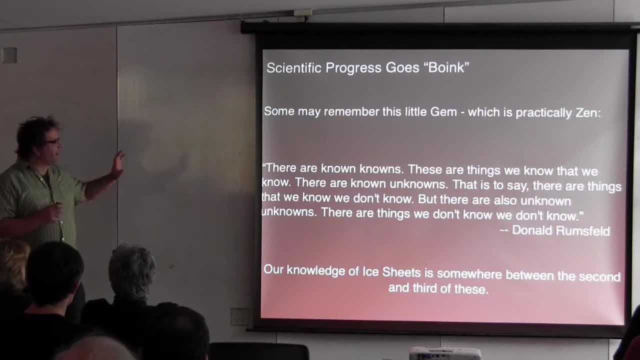 So he could have said: there are facts, questions and surprises, And people would have walked away knowing what he was actually talking about. This is an unknown. unknown Just our knowledge of the polar ice sheets, the great ice sheets of Antarctica and Greenwood. 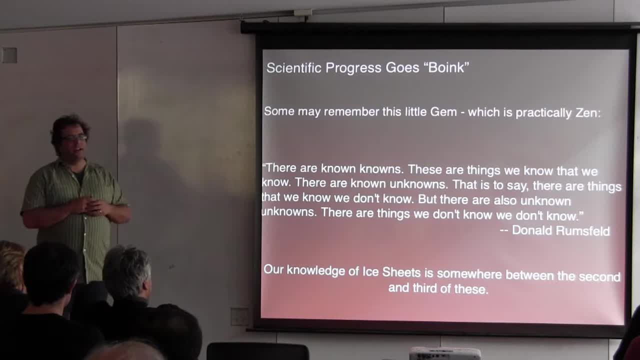 are kind of somewhere between the second and the third of it. We've got some facts, but we've got an awful lot of questions And we've got an awful lot of surprises Every time we look at an ice sheet closely. Richard Elliott, Penn State, has said this before. 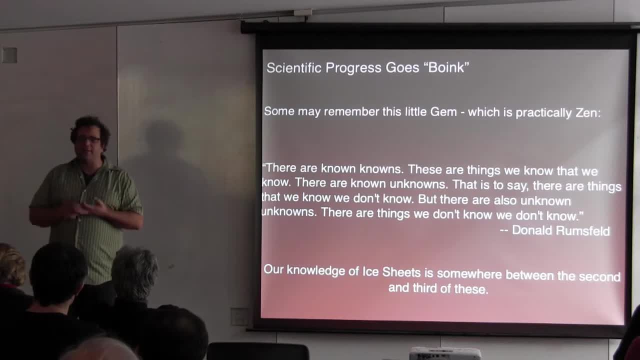 every time we look at an ice sheet closely, we find something new that surprises us, Which means that we don't yet fully understand the ice sheets And there's a lot more research to be done. So that's the kind of state of knowledge just now. 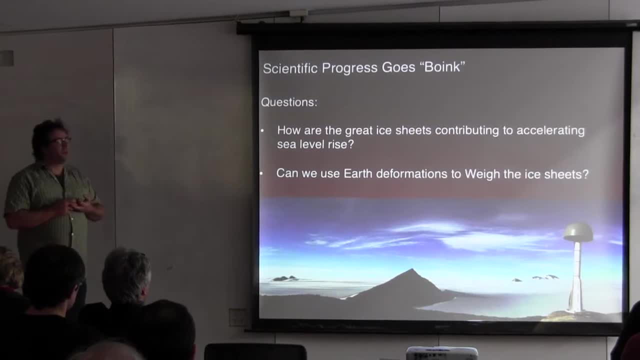 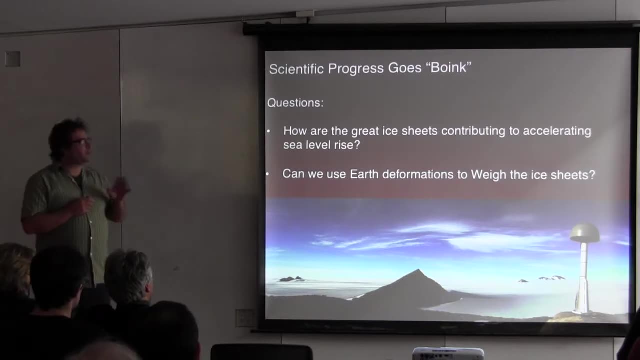 So some of the known knowns or some of the known unknowns, or the things that get me out of bed and get me doing the work that I do: How are the great ice sheets contributing to accelerated sea level rise And can we use earth deformation to weigh the ice sheets? 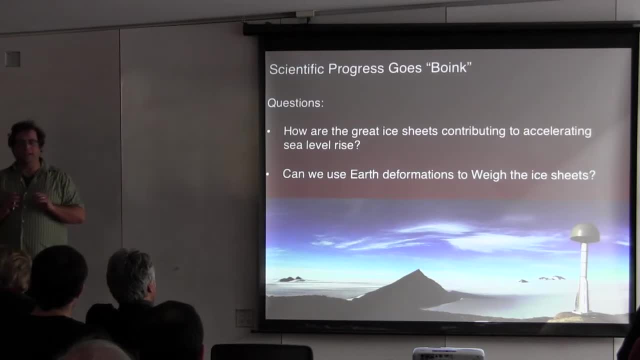 So I'm going to talk through this. There are two or three different techniques that we put together to answer these questions, But this is just a really photogenic GPS site that we installed in southern Greenwood. So I'm going to cover GPS, the global positioning system. 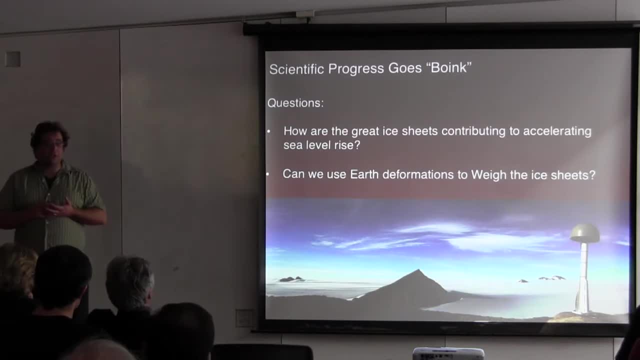 I'm going to cover stuff from a satellite system called GRACE, which is the Gravity Recovery Climate Experiment, And I'm going to cover some of the stuff that actually Andrew, who is a student of ours who has a PhD, will work on with digital elevation model differencing. 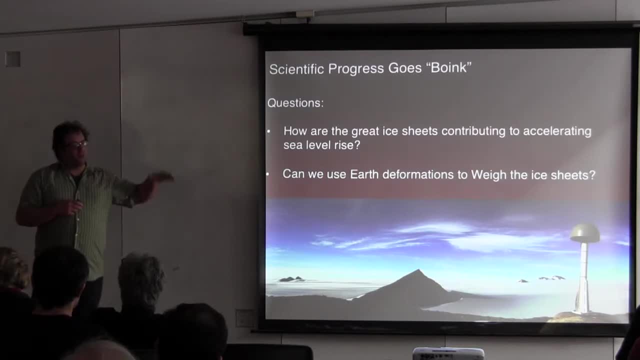 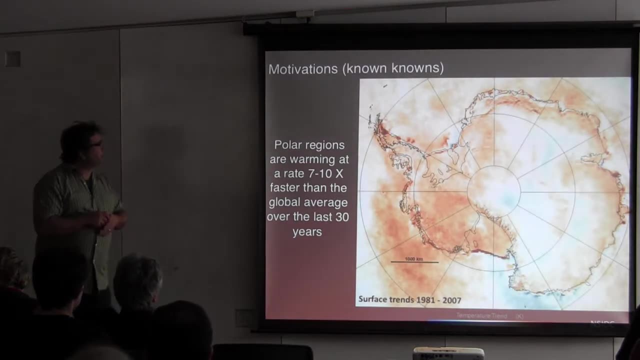 which is getting representations of the topography of the earth and watching them evolve through time, and what that tells us about the earth and about ice So known knowns, some facts, some motivations. The polar regions are warming at a rate 7 to 10 times faster than the global average over the last 30 years. 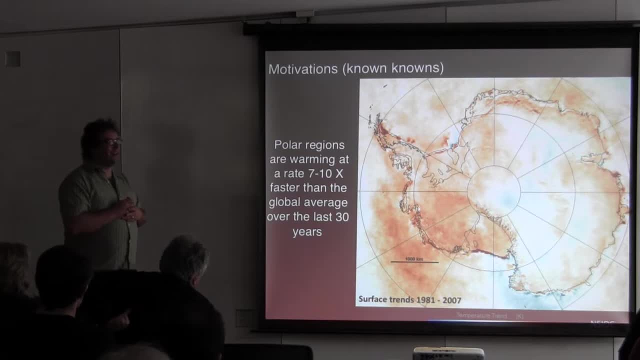 Just now we've had cold weather down in North Carolina and, oh you know, the sky is falling. the sky is falling. climate change can't be real. It's been 15 to 20 Celsius warmer than average for January and February in the Arctic. So the great cold that we're getting down south is rather nicely balanced by great warmth that's occurring up in the Arctic. The January sea ice in the Arctic is about 80% of the size that it should have been, Compared to the last 30 years. 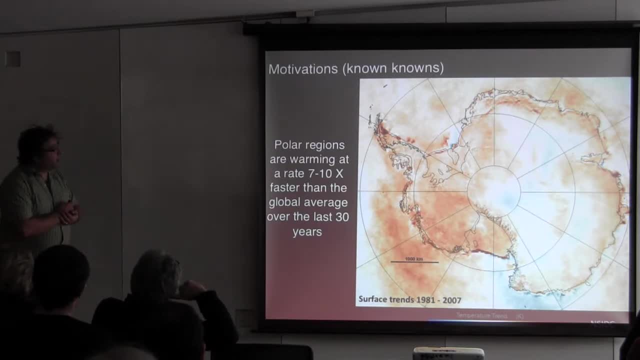 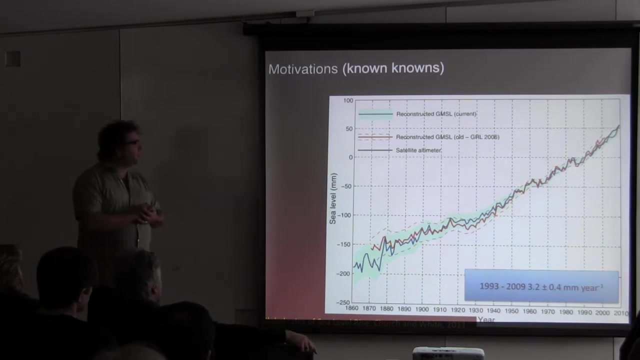 So sea ice is disappearing In the Arctic. in the Antarctic it's not such a problem, But in general the Arctic and Antarctic regions are warming faster than anywhere else, Sea levels going up. Sea level was going up about a millimeter per half per year. 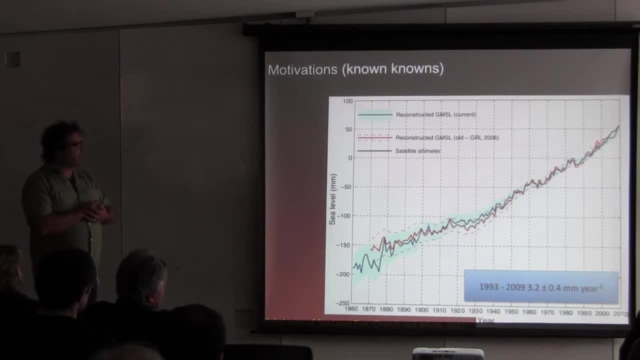 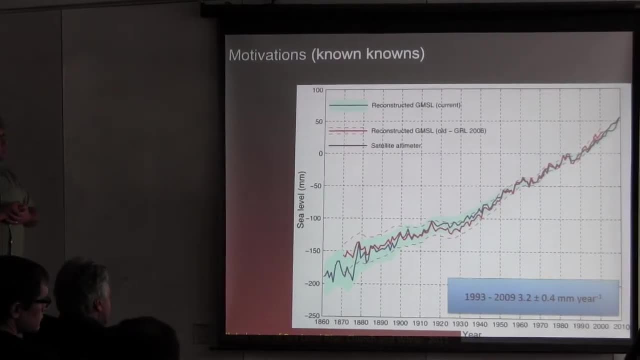 But the 1993 to 2009 average- and this number is getting slightly larger now- is 3.2 millimeters per year, So a tenth of an inch or so, And that acceleration has generally been the last you know two to three decades where that's occurred. 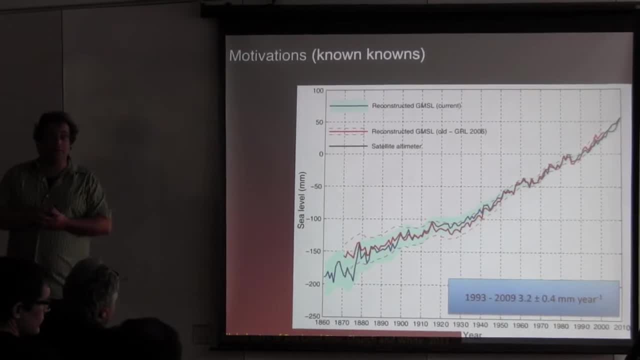 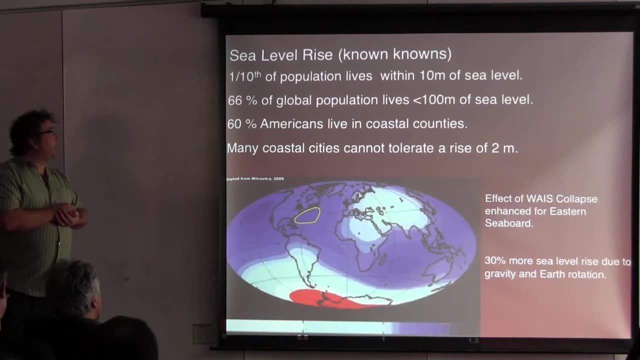 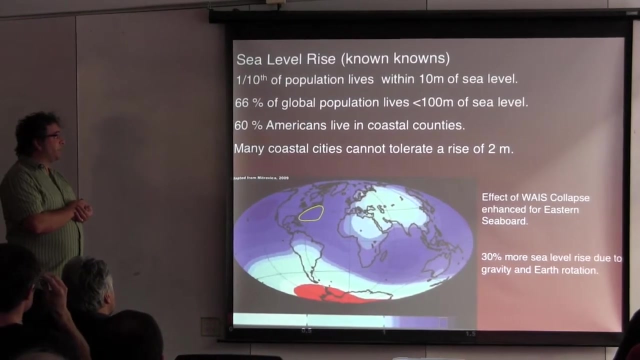 We get that from time gauges and we get that from satellite activity around the world. Why do we care that sea level's going up? One tenth of the Earth's population lives within 10 meters of sea level. 66% of the global population lives within 100 meters of sea level. The sea level's not going to go up that high. The by far the densest populated counties in the USA are coastal And many coastal cities- London would be a good one, the Netherlands, New York City, Washington DC or somewhere. 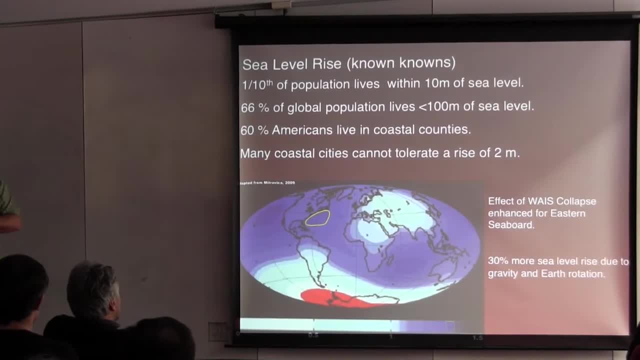 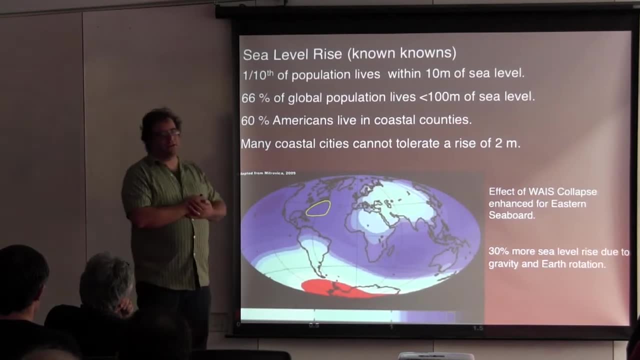 we don't worry about that. so much can't really tolerate a rise of two meters. Two meters aren't enough, Isn't on the cards for the next 100 years or so. But take the 200 years, 300 years: two meters, it's going to be something which is probable for a lot of coastal cities. 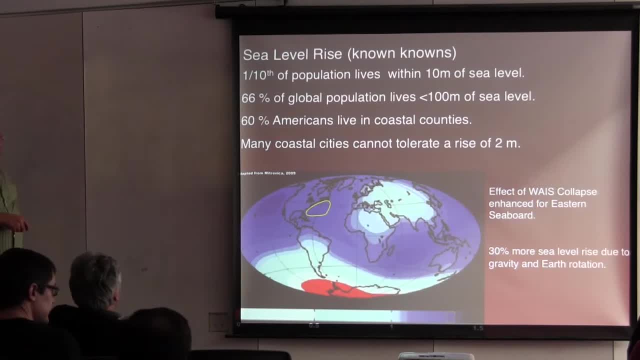 And we were talking earlier about what happens when an ice sheet collapses. Well, if you remove ice in Antarctica, you've got some things, so the land bounces back up, which displaces water, But you also have a gravitational effect. So just now, the mass of ice in Greenland or Antarctica pulls water together just due to the gravitational effect. 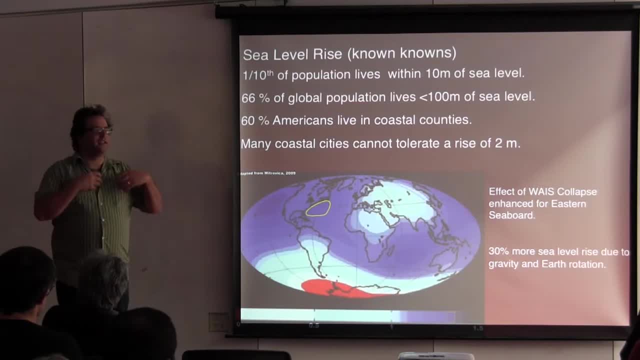 If you remove that ice sheet, the gravity drops and that water flows away. So close to an ice sheet, the immediate response of the ocean when ice disappears is that sea level drops. But Jeremy Trevika, who's at Harvard, has done some really cool modeling of this and he's found that if the ice disappears from west Antarctica, 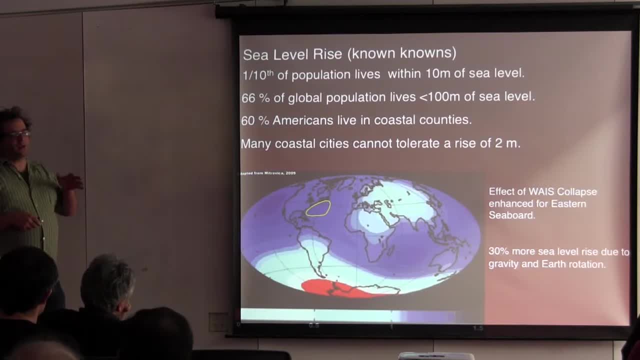 then stuff on the eastern seaboard is going to go up between 30% and 50% faster than the global average. So if it goes up a meter on the globe it'll go over a meter 30 to a meter 50 on the eastern seaboard of the USA. 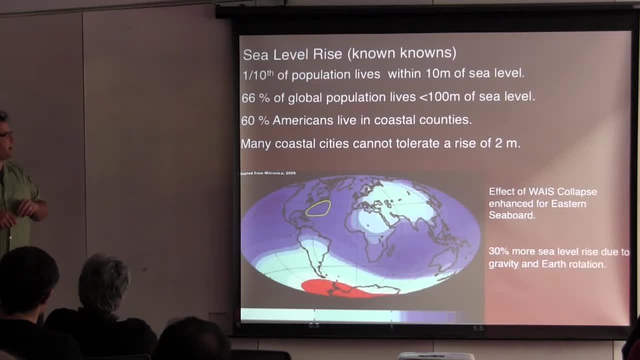 If Greenland were to disappear or a lot of the mass were lost in Greenland, that would kind of be reflected down in Southeast America. That's called a sea level fingerprinting, But it basically means that you can't just take the global average and 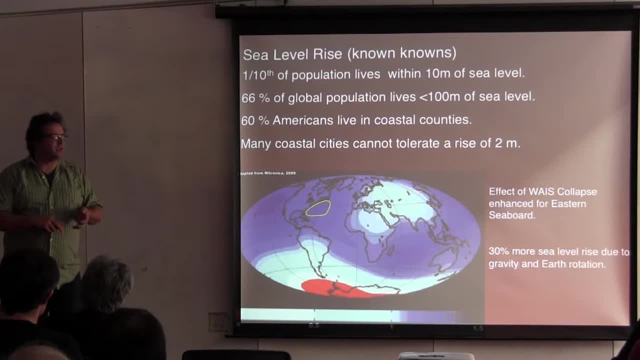 oh, sea level's going up here. sea level's going up there. There's lots of complications with gravitational feedback, with gravity, with the crust adjusting to the different loads. They generally mean that the east coast of the USA is not somewhere particularly wonderful when it comes to sea level rise. 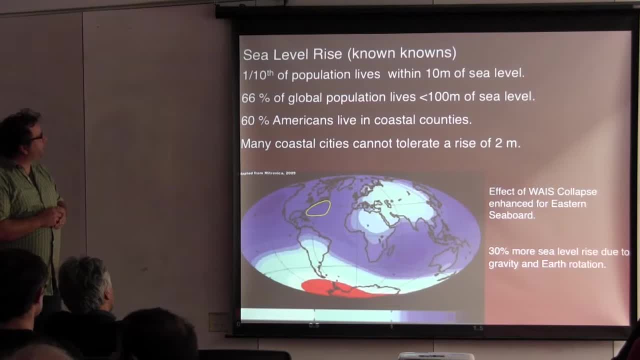 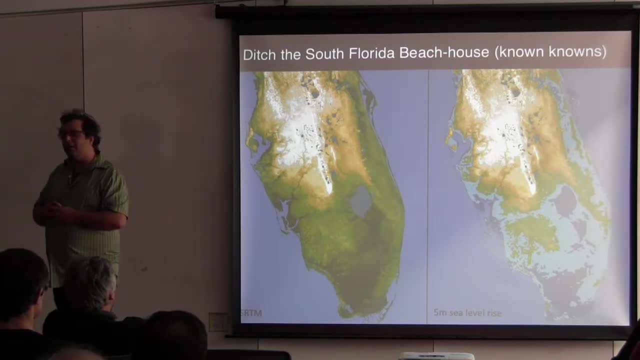 as it's occurring on the west. I sometimes do this to annoy people. Ditch the south Florida beach house. Ditch it If you're going to buy one. it's not a good idea. It's not a good investment. This is five meters of sea level rise, which will take you all up through the other place. 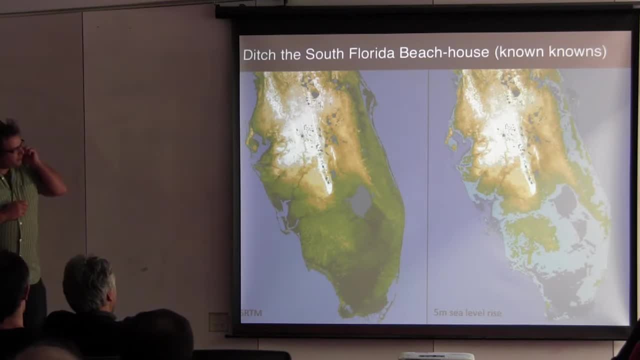 Miami's gone. Downtown Miami's only about two feet, three feet above sea level. Two, two and a half feet above sea level, So we don't even have to get a meter of sea level rise and your property values for the financial district in downtown Miami go through the floor. 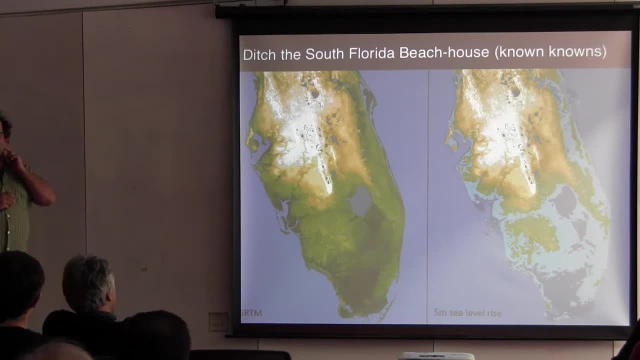 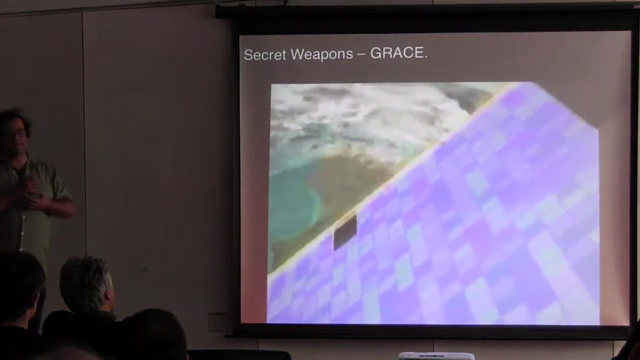 So, again, not your greatest investment opportunity for those who are young, and you might even want to hold onto it If you're getting along. NASA disappears as well when sea level goes up. in south Florida, We do have some secret weapons for answering what's going on with sea level. 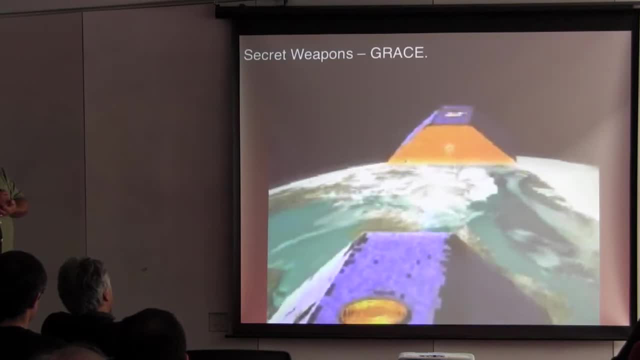 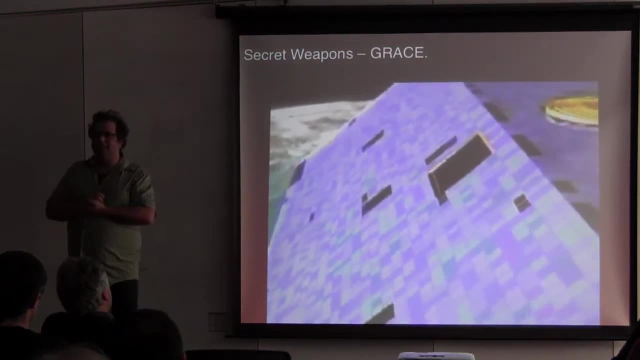 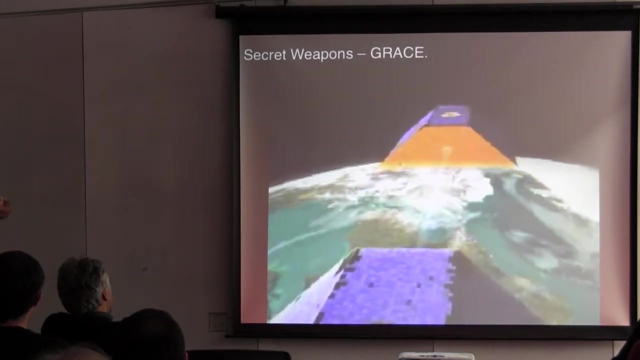 what's going on with ice? mass changes in the polar regions. And this is the schematic cartoon of the GRACE satellite pair: Two really weird looking trapezoid satellites that follow each other. They're separated by about- I think it's about 200 kilometers. 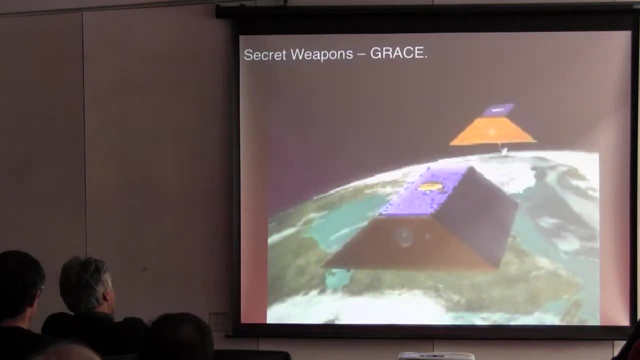 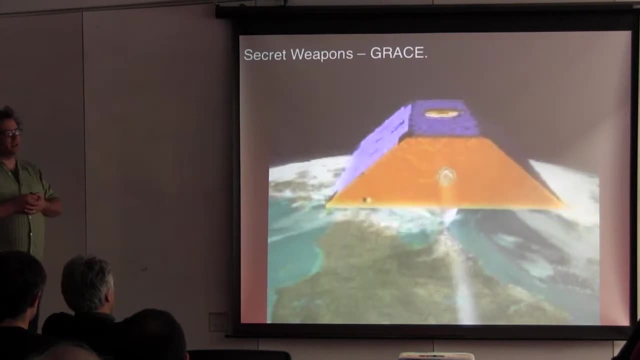 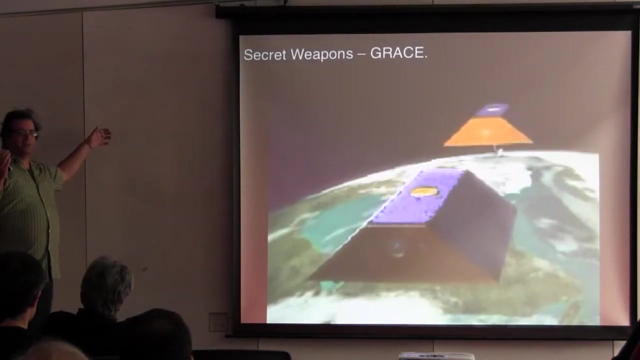 And they fire a radar beam between the two of them. And what they do is, as you measure the distance between the two satellites, as one of them goes over the mass, it gets pulled forward a little bit And the other one, which is further behind in the orbit, stays back. So you get the distance that increases between the two satellites. As that second satellite passes over the mass, it speeds up a little bit and catches up with the first satellite. So you have these two satellites that are kind of bouncing backwards and forwards. It's like the Tour de France. 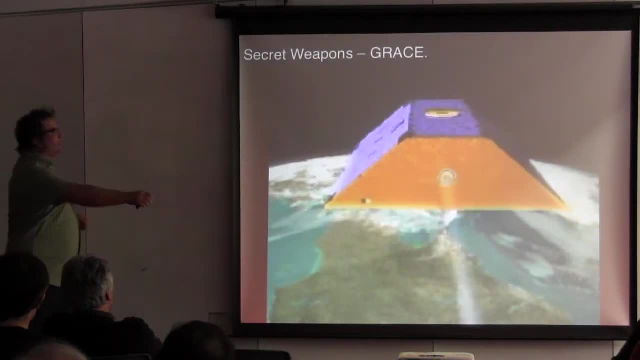 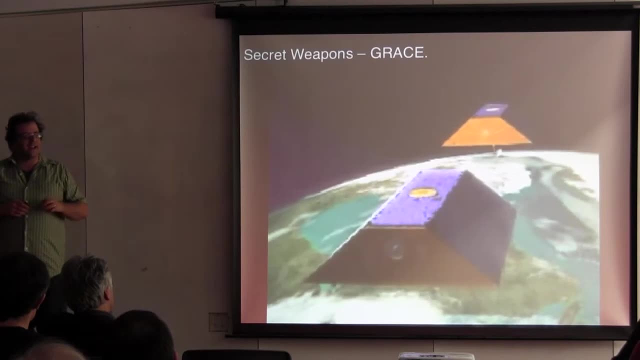 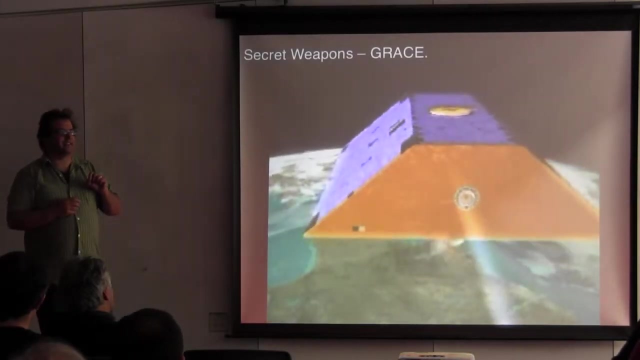 You know, a person goes out in front, sometimes they catch him up, sometimes he takes off and sometimes they catch him up again. But by measuring the distance between the two satellites you can exquisitely decide how much mass is underneath the satellites. 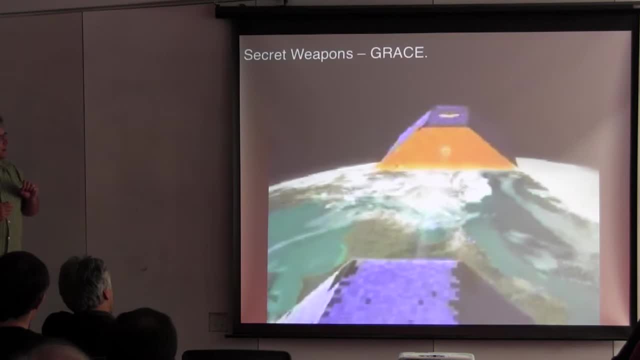 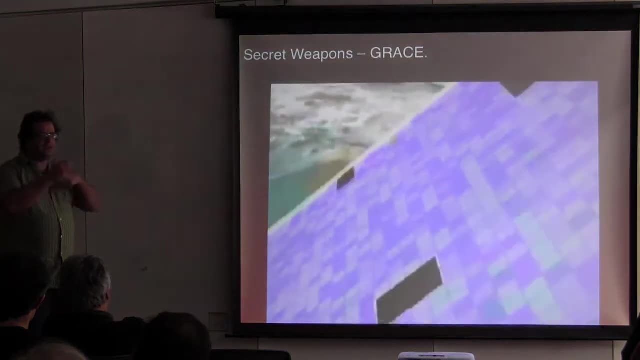 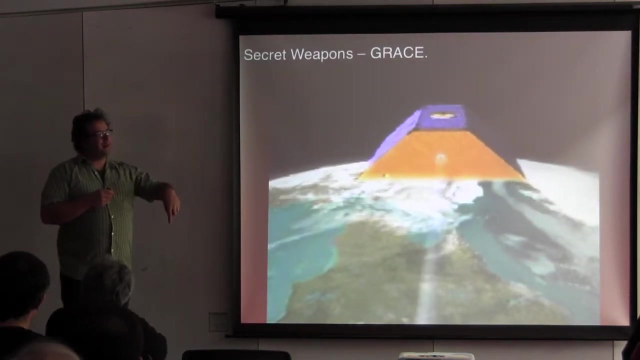 I mean, it's a beautiful, beautiful, elegant system, But it can only tell you the mass underneath you. Now what happens is it orbits about. once a month It goes over the same place. So once a month you get a measure of what the mass is beneath the system. 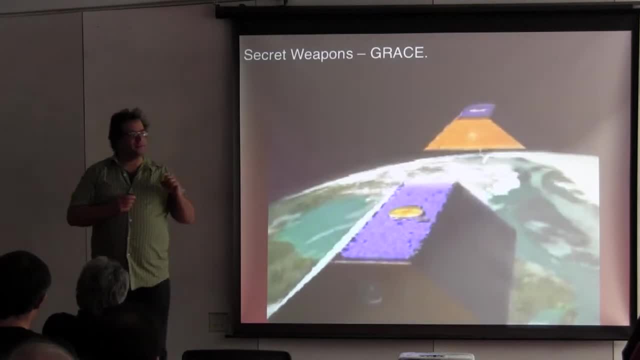 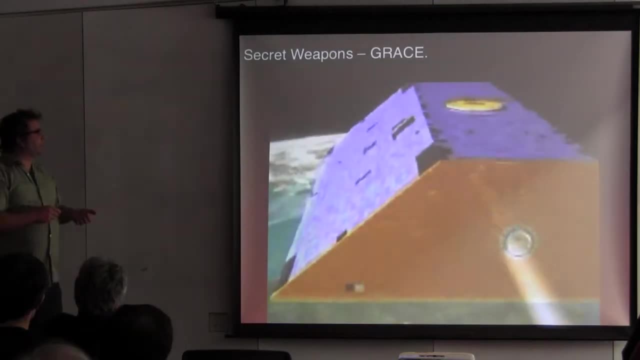 So through time you can see if there's mass changes, And this has become really useful for measuring changes in space. We're interested in water, basically Water in any of its forms, be it in rivers, in oceans, in lakes. 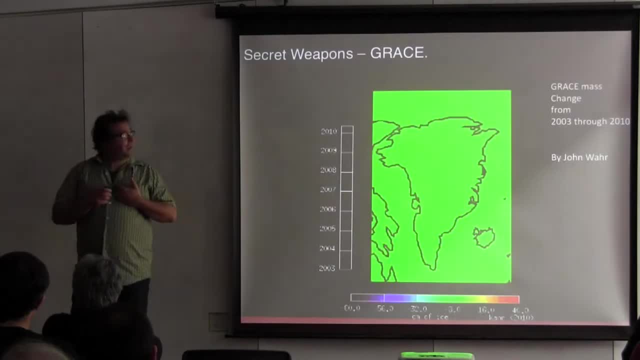 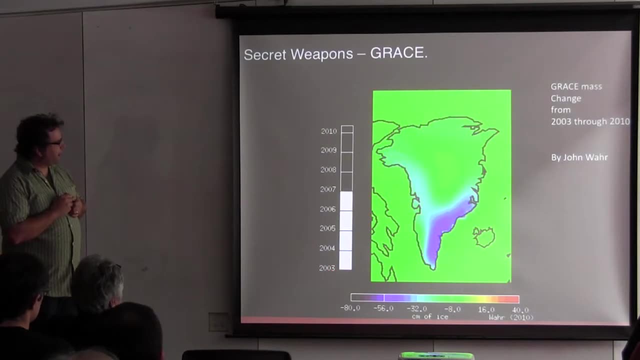 or, as we're interested with ice. So this is what GRACE sees between 2003 and 2010.. And this is changed into centimeters of ice being lost, So you can see that occasionally you have some ice being added, but wow. 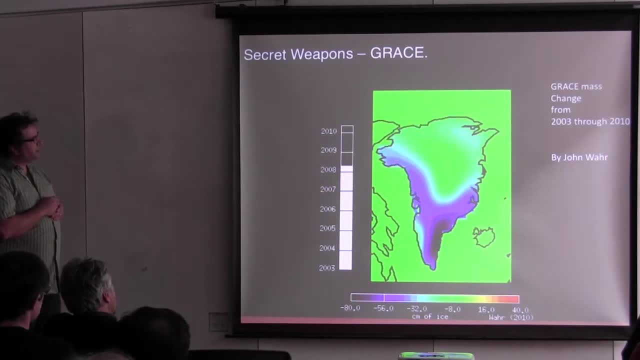 2005.. The southeast of Greenland really starts losing mass, And that up through 2010,. that mass loss is spread up into the northwest of Greenland. What we have to decide is: what's causing this mass loss, Because this exquisite sensor is measuring it, but what's causing it? 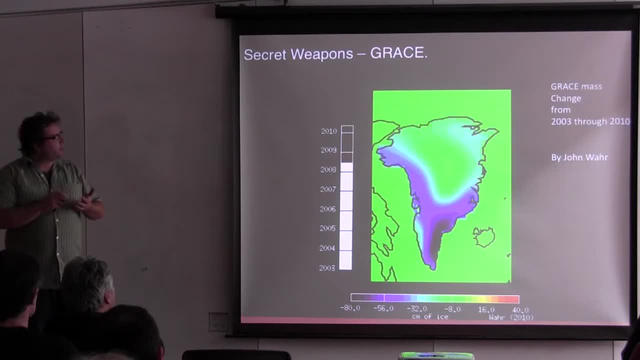 And you've got two things going on: You've got ice, You've got ice moving faster into the oceans And you've got changes in the amount of snow and ice being deposited on the ice sheet. So we call that dynamics. Is the ice changing its speed? 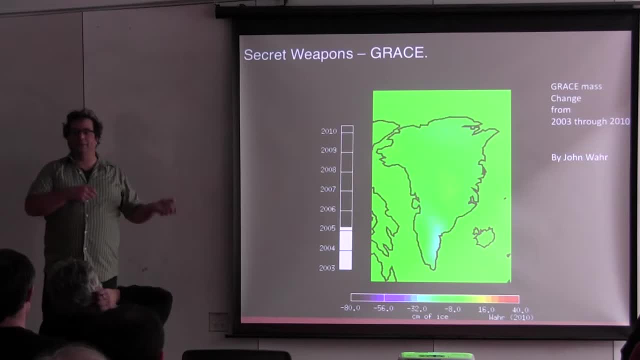 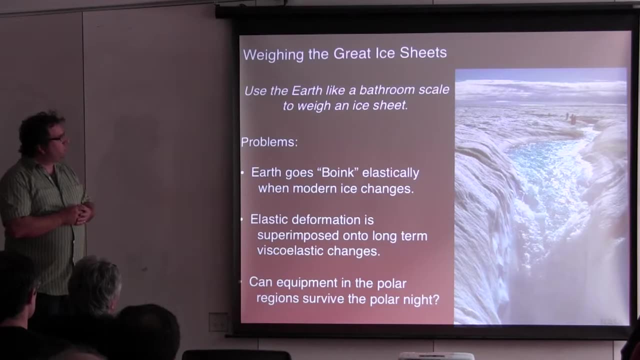 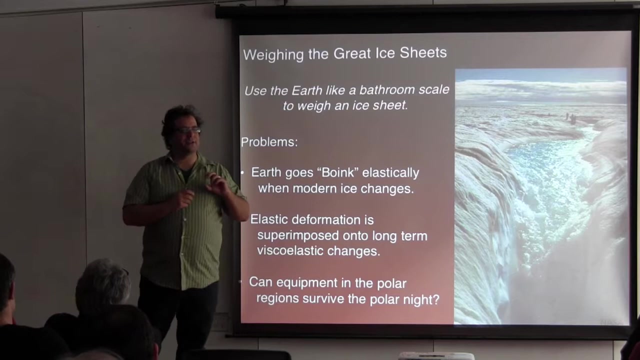 And you've got surface mass balance, which is the amount of snow that's added and removed from the top of the ice sheet each year. So with that we can kind of weigh the green ice sheets. But there's a problem: Earth does actually go boink as you add mass and take mass away from the ice sheets. 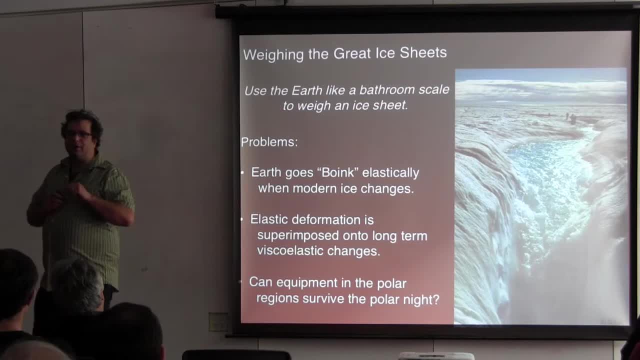 Underneath the ice sheet, the mantle and the crust response And that's a mass that Grace can tell you the mass changes but can't tell you what the mass change is caused by. So it can be a mix-up of ice sheets. 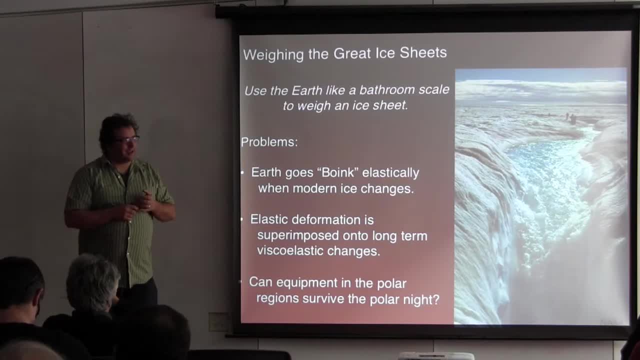 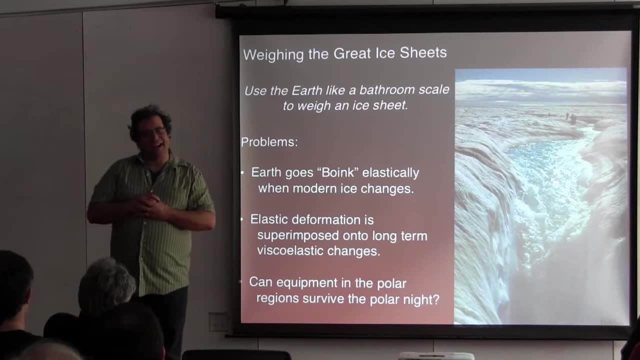 Ice changes and mantle changes, And so we have to correct this sensor through time using pretty complicated models, which is what Sam's going to get into And it's going to cause you time. It's going to take your entire PhD. I'm sorry, but it's going to take your entire PhD to sort it out. 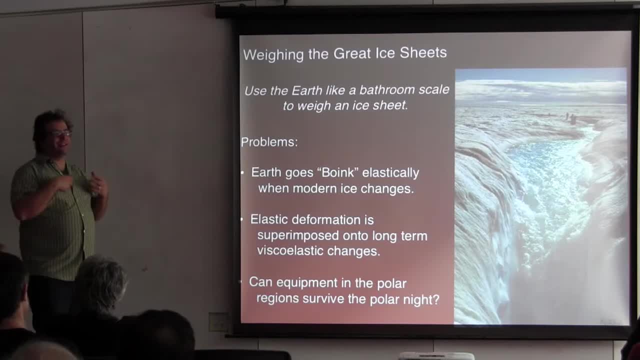 So you have two sorts of signals. You have the sort of signal that reacts. now I'm going to stand here. The Earth is going to bend underneath me- Maybe not too much, but the Earth is going to bend underneath me. But if I stand here long enough, I'm going to sink further and further and further. 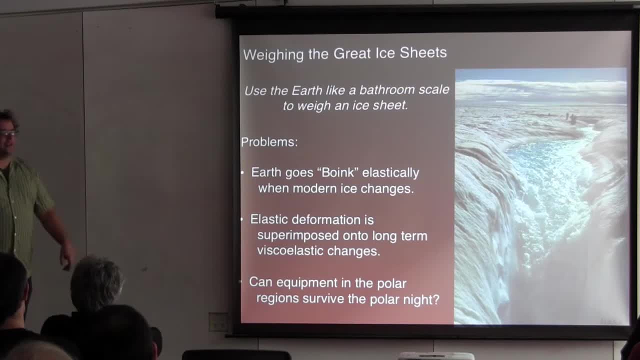 and the mantle is going to move away too. If I remove myself, the crust is going to come back up, And what we found is it's going to come up pretty fast, And then the mantle, which is very much denser than ice. 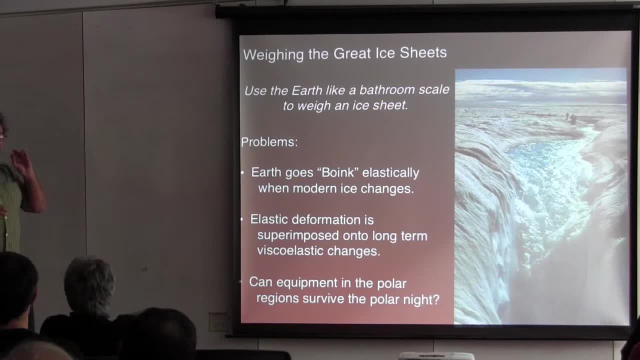 is going to fall back into that space And that's a mass change. And Grace can tell you that those things are occurring, but it can't tell you this proportion is caused by this and this proportion is caused by that. We're going to look at that elastic deformation and say, year after year after year, 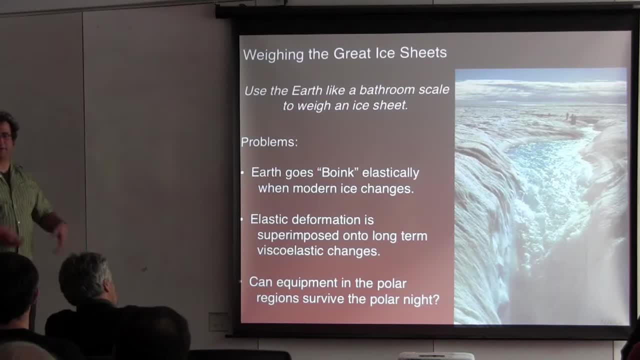 we can see ice being added and taken away by surface mass, balance and dynamics. What can we measure with GPS on the ground in these places? And then, how do we take those elastic signals, those long-term physical elastic signals, put them together and actually get a handle on what the great ice sheets are doing? 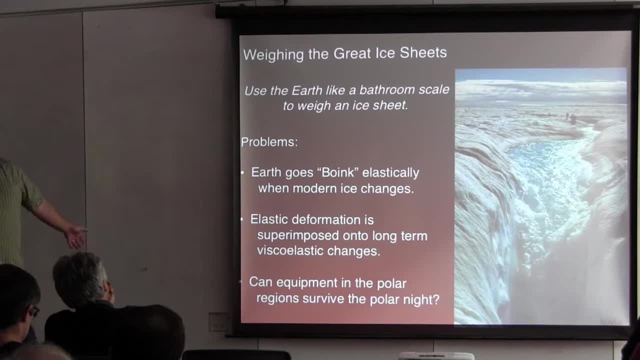 The other thing to do. that is, we need to install GPS everywhere. We've installed 55 GPS in Greenland And as of last week, we're at about 55 GPS in Antarctica on bedrock. And then we need them to record every 15 or every 30 seconds for years and years and years. 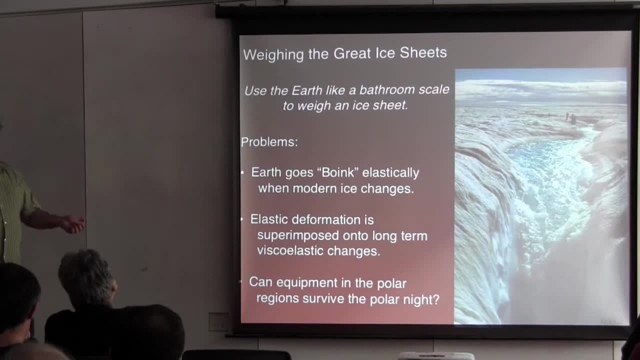 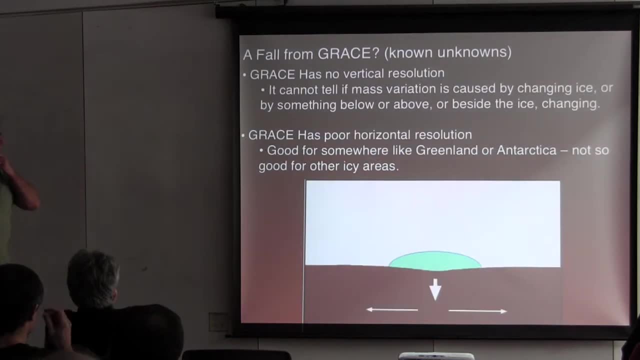 before we can get a good handle on it. And your issue there is: it's dark in the winter. Where do you get the power from? I'll go back to that in a second. So grace is this wonderful thing, But do we have a fall from grace? 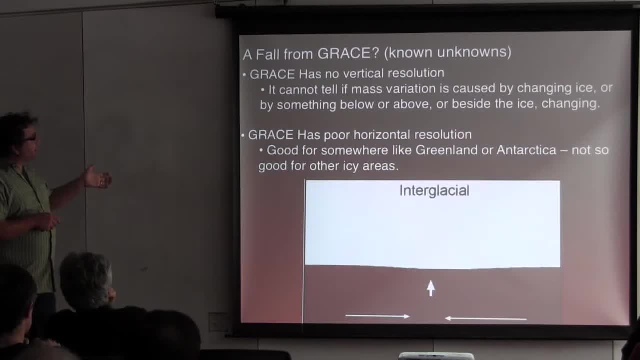 We know there are questions about it. It has no vertical resolution. All it can tell you is beneath the satellite, mass is changing. It can't tell you where or what directly below you that mass is, So it can't tell you if it's caused by changing ice or something below. 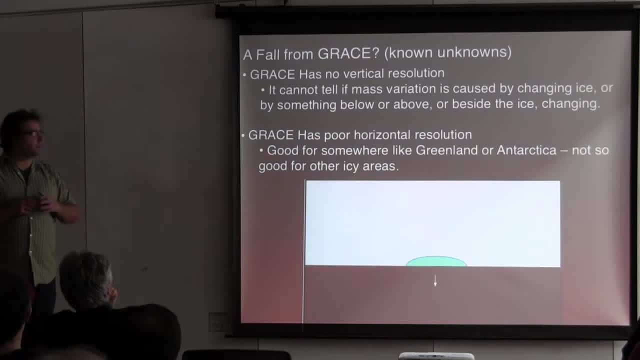 above or even beside the ice, changing. That's called lineage. It's also got pretty poor horizontal resolution. I showed you that map of the blue spreading out over Greenland That's made up of pixels which are maybe about 300 kilometers across. 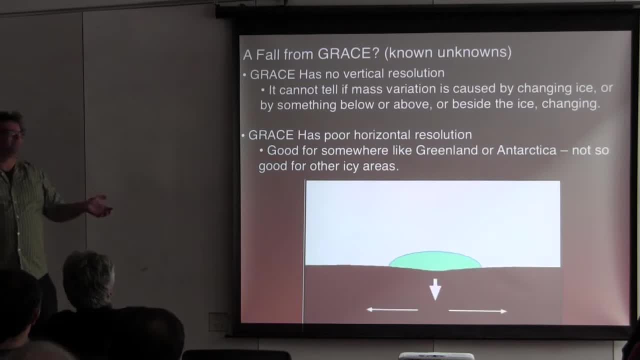 So you know, half from here to what's 300 kilometers. Here to Buffalo, Would that be 300 kilometers? Yeah, I mean 120, 150 miles, So a pretty big coarse resolution. Temporally they're really fine. 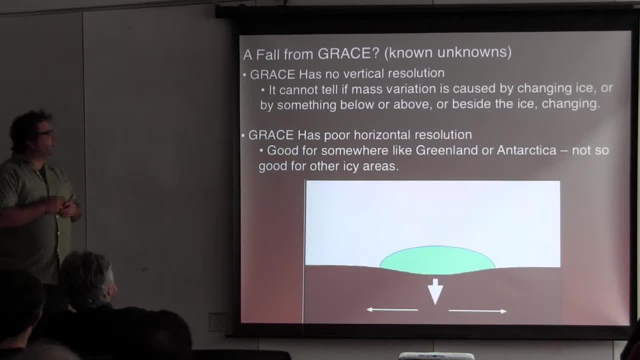 But spatially they smear things out into the big, big areas, Which I see it's good for somewhere like Greenland or Antarctica, but I'll show you some caveats to that later on. It's definitely not very good for really small ice masses. 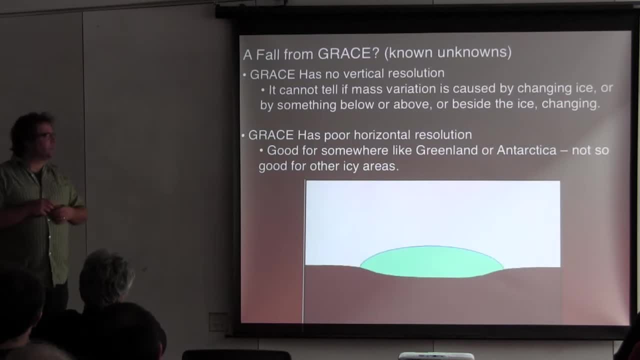 which, when you add up the really small ice masses, they actually have an appreciable signal too. So the little diagram down at the bottom here is just a little, a little movie animation of ice building up during the last glacial maximum. 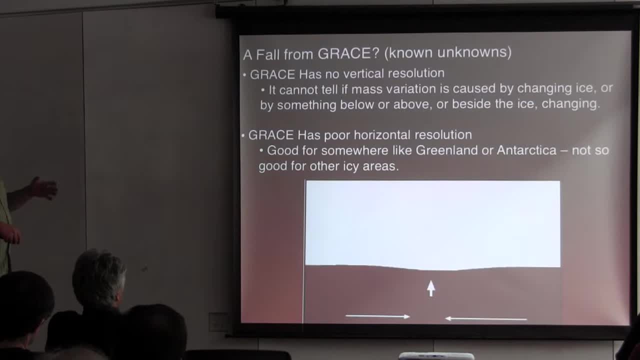 And, as that happens, the Earth is pushed down As the ice disappears and we go into an interglacial, or you know, a warming event with the ice. here's the ice building up, the mantle moves out of the way and the crust moves down. 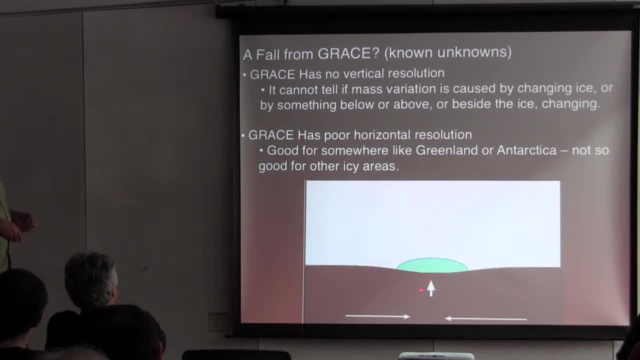 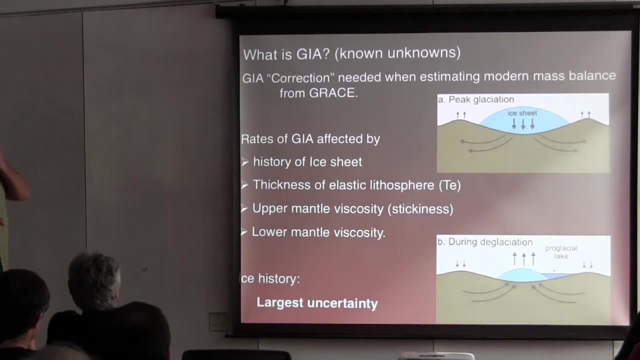 And then, as it shrinks, the crust moves back up and the mantle moves in. We put GPS kind of around the edges, All right. So what is GIA is Glacial Isostatic Adjustment, which is the correction we need to put to that gray satellite. 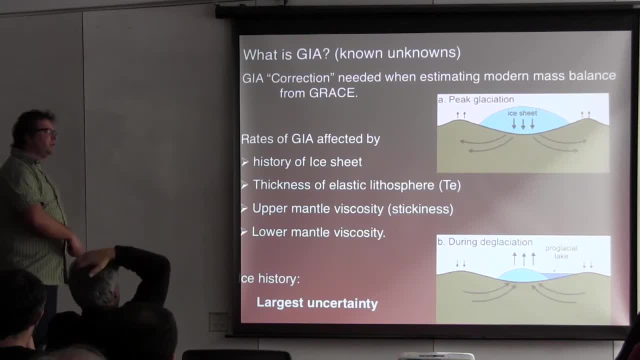 to get a real handle on what's happening now and what signals we're getting now are due to the past. GIA is affected by the history of the ice sheet: where the ice sheet was, how long it sat there, how long it took to disappear. 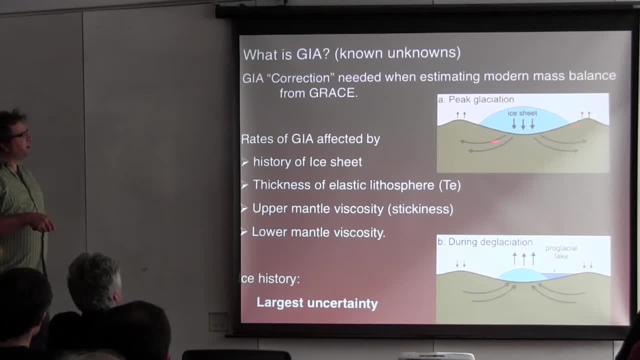 It's affected by just how thick the elastic part of the lithosphere is. It's really affected by the upper mantle viscosity, or how sticky or fluid the upper mantle is, how easily it can move out of the way, The lower mantle viscosity. Of these, though, the largest uncertainty comes back to 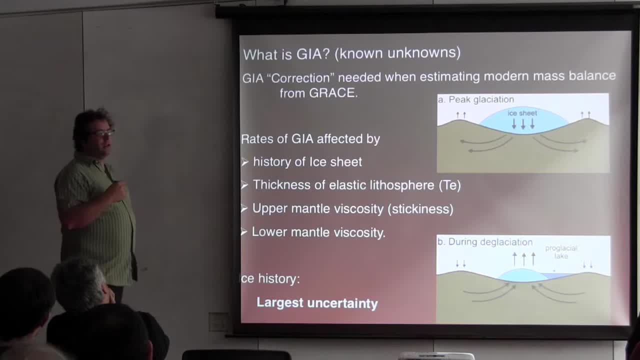 we don't really know well where the ice was at what time in the past. Ice sheets have this horrible when you put a glacier somewhere and it comes forward and leaves you this beautiful record and then retreats and you get this beautiful record. You can go and do proxy stuff. 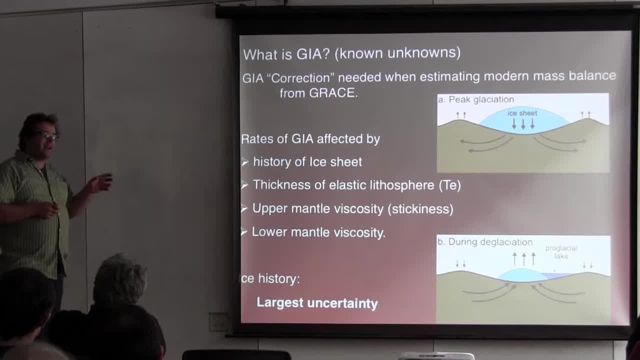 You can go to paleoplanetology on all these records. They have a habit of then re-advancing and going over the top of all the signals that you wanted to record. So you can. it's very hard to get long-term signals. 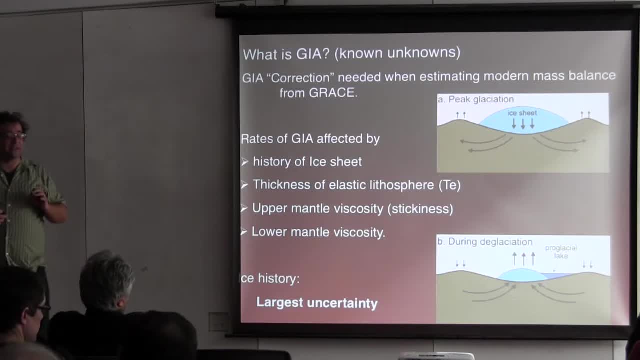 and what an ice sheet has done around the edges or even in the middle of it. People say: we've got all these beautiful ice cores. We do have beautiful ice cores. We've got about 20 of them in total For something you know: the Antarctic ice sheet. 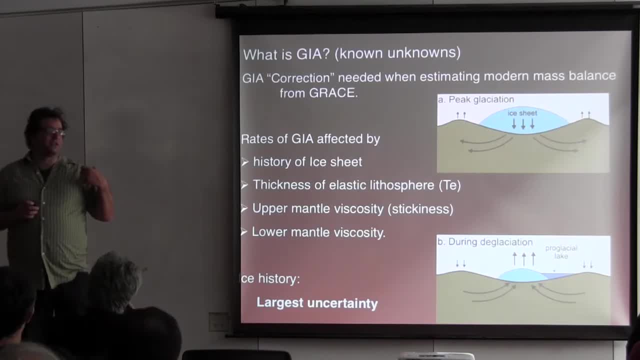 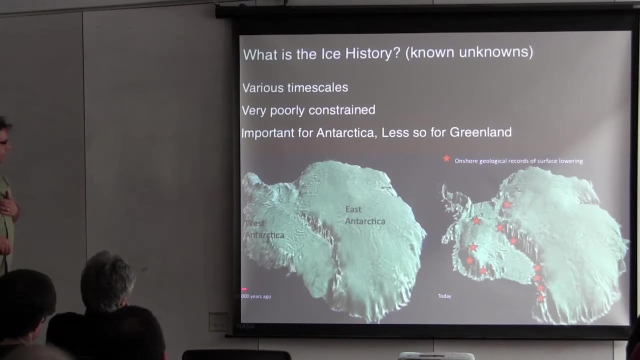 is the size of the USA plus Mexico. So we've got 20 little points where we can tell you what happened there, what happened everywhere else. We're still trying to figure that out. Again, one of the- no one knows This is a really rather crude now reconstruction. 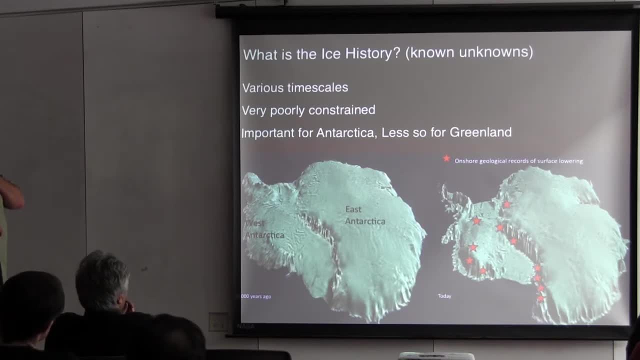 of what Antarctica looked like 20,000 years ago. This kind of reconstruction changes on what seems to be a daily basis. More and more recent publications are saying that the amount of ice that East Antarctica and West Antarctica had 10,000, 20,000 years ago is less and less and less and less. 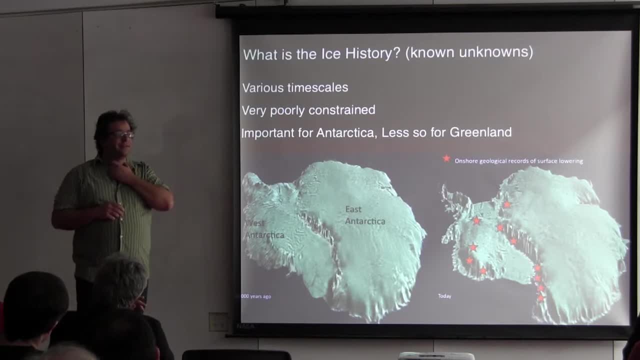 Antarctica doesn't seem to be responsible for so much of the sea level change that we can see from paleo records of the last 10,000 years as we thought. But this reconstruction, for example, was constrained with 1, 2,, 3, 4, 5, 6,, 7,, 8,, 9, 10 data points approximately. 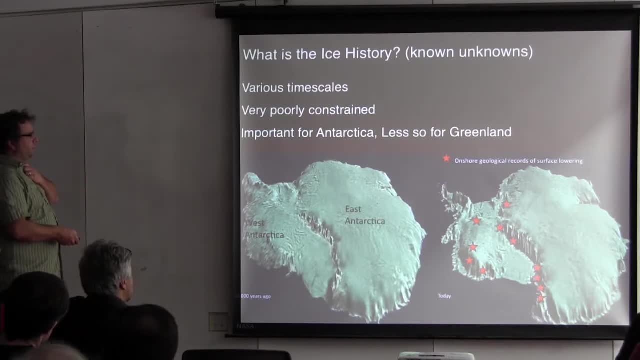 And we now know that these four are wrong. So we've modeled all of this, all of this mass change here in East Antarctica and all of this mass change over here in West Antarctica Based on that, And that's the issue in Antarctica. 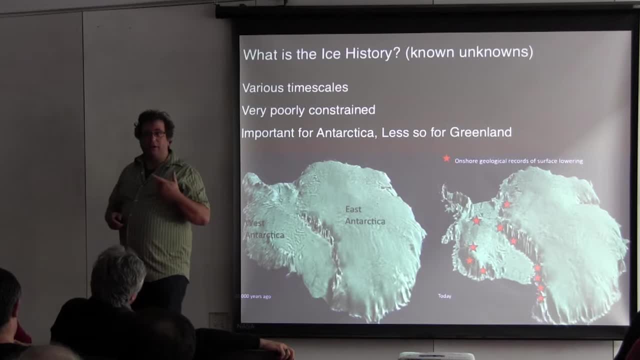 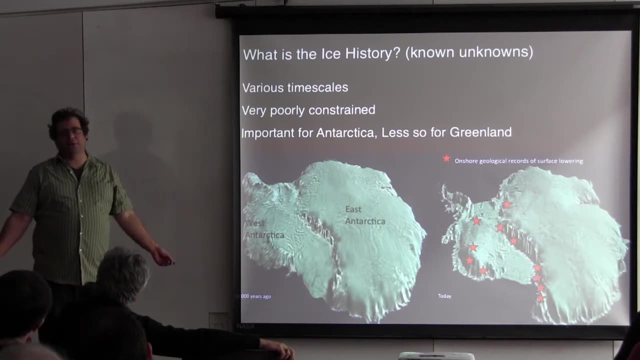 Where are you going to get these records? Are you going to get them from these 20 or so ice cores, Or are you going to get them from bedrock? Now, USA plus Mexico, bedrock's Delaware- 2% of the continent isn't covered by ice. 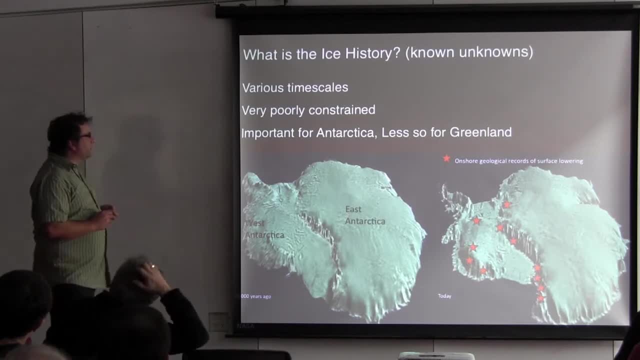 So there's very limited places where you can actually get these records, But we're trying. We're getting better. We think most of the ice change is actually now through here in the Southern White Isle Sea and a little bit through here in the Southern Ross Sea. 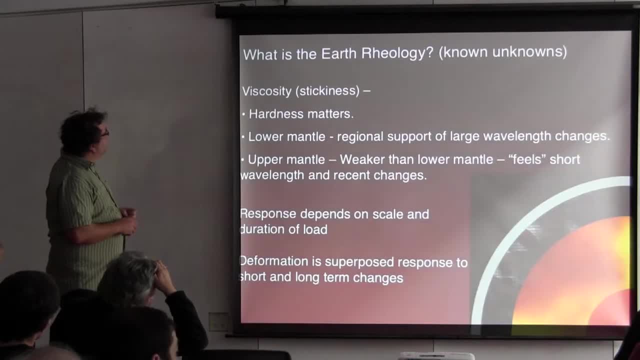 Places where we actually can't get very many proxy records, unfortunately. Then you have. so you have for GIA. you have the ice history and then the Earth's mechanical properties. We call that the rheology, Another known unknown, And we're looking at the stickiness of the upper mantle. Part of the matters. When you have very big changes they're felt by the lower mantle, But the upper mantle it feels a lot of stuff that the GPS would more easily feel. The risk of loss of the Earth depends on the scale and duration of the load. 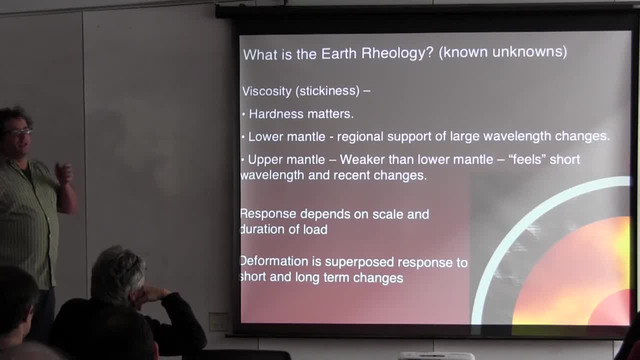 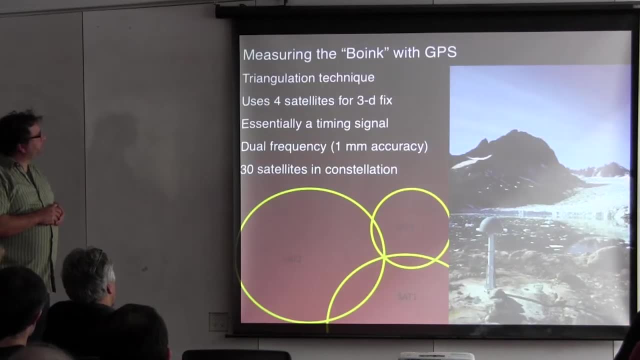 how long the ice sits there. And those responses for the long-term changes and the short-term changes are superposed on top of each other, So measuring the point with GPS. Most people now are pretty familiar with what GPS is. It's a military satellite system. 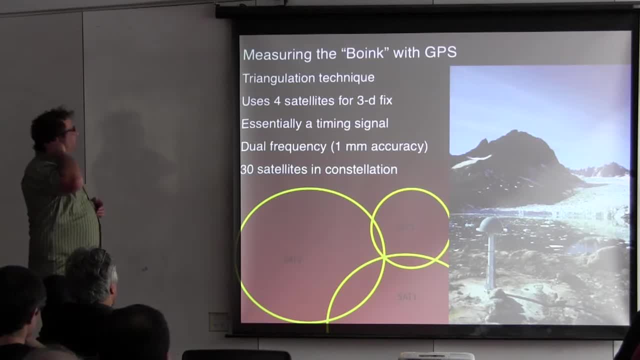 The US Air Force started launching it in the late 80s and early 90s. It uses triangulation. You need four satellites in view at once to get a three-dimensional fix. This is a schematic. You've got satellite twos here, satellite threes here, satellite one. 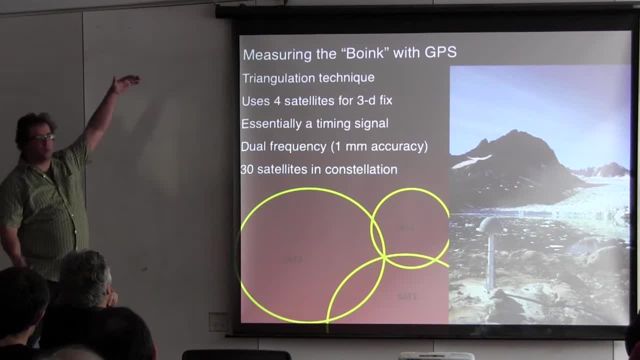 You're guessing that if you're actually in a four-satellite, you get an idea on your timing and on which side of the Earth you're actually on. We use things that you don't get in your car. Cars are typically about 10 grand each. 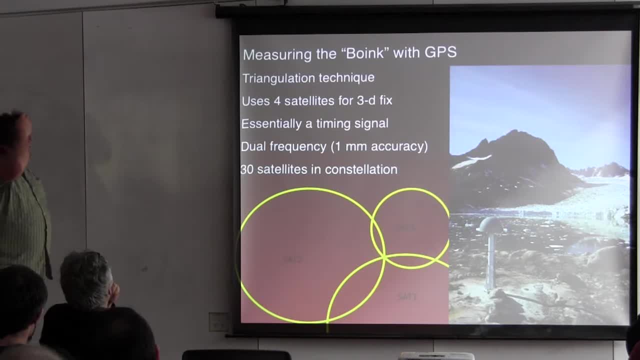 So 55, though you're starting to add up, They're good to a millimeter accuracy. The way I like to illustrate that is if you dropped a quarter and it got lodged in the sand and we went and positioned it, we could say it's there. 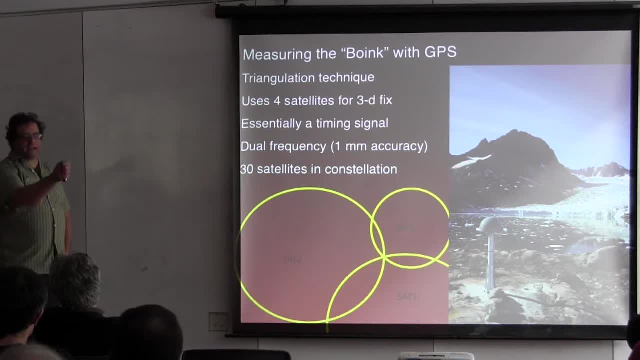 If we came back 10 years later and we went to the same place, that quarter wouldn't be there. It would have moved, because the plate has moved. We're good enough to measure. okay, there's the edge of the quarter there. 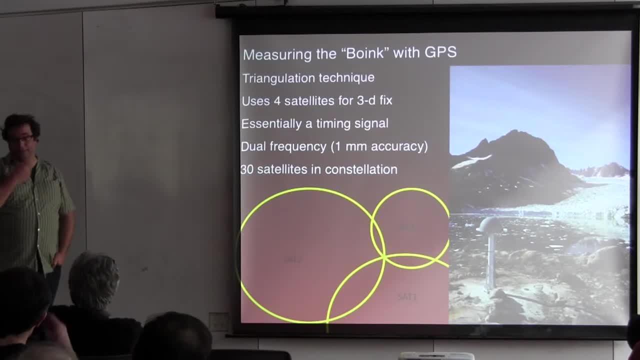 there's the edge of the quarter there. That's how far the plate has moved in the intervening 10 years. So these are- yeah, they're stupidly accurate. They're very complicated to deal with and they're very expensive to build. 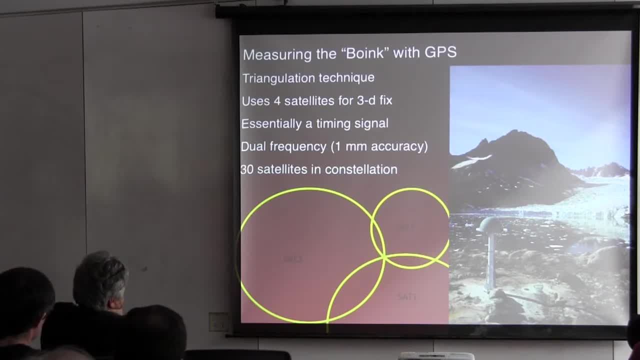 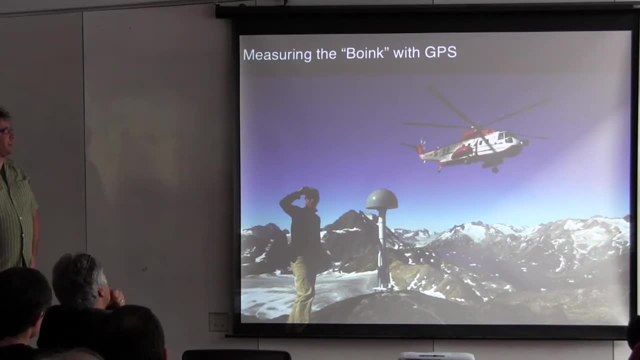 but we do get to go and vandalize some really beautiful places. How do we install them? Of course, the S-26 helicopter is a pretty good start. It can carry the number of batteries in northern Greenland and in southern parts of Antarctica. We have stations which have 26 deep cycle marine batteries like you put on your boat, So they're about 60 or 70 pounds each, And I was basically hired to carry batteries up mountains. That was my PhD and master's. It's cold work, it's hard work, but again we get to go see beautiful things. 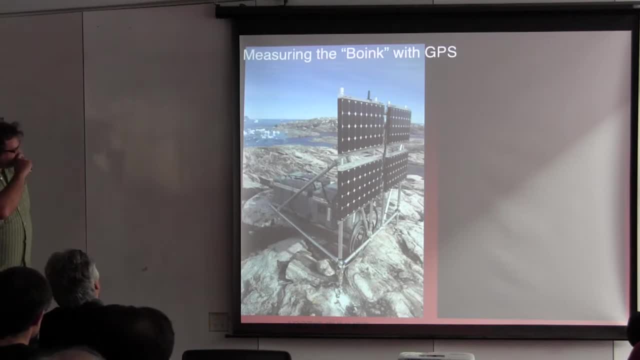 This is a typical system. This is in eastern Greenland. We've got four solar panels, a bank of batteries here and sometimes we'll have a wind generator, And the reason we've got so many solar panels and so many batteries is this is the Arctic Bay. 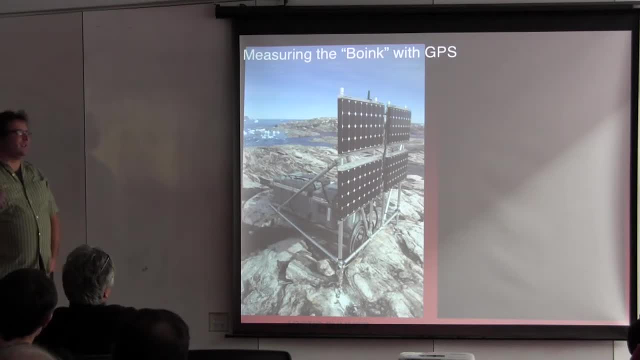 24-hour sunlight. we're getting loads of sun coming in. We can do real-time communications with these things. I can look them up on my phone And this is an outlet. Not so much when it comes to solar power. It's dark, depending on the latitude, for up to six months of the year. 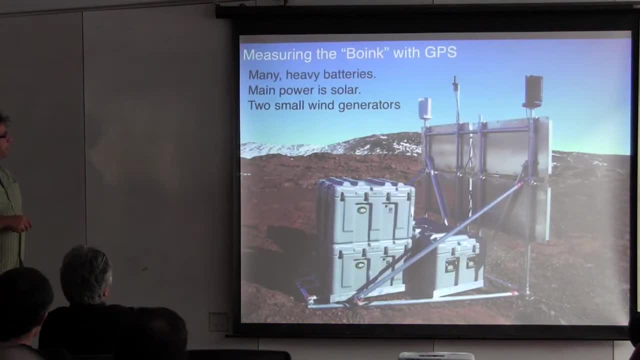 But we've been very successful. As I said, many very heavy batteries. This one will have 12 batteries in here and 8 batteries in each of those, So a couple of little wind generators which are experimental and have turned into the bane of my existence during this project. 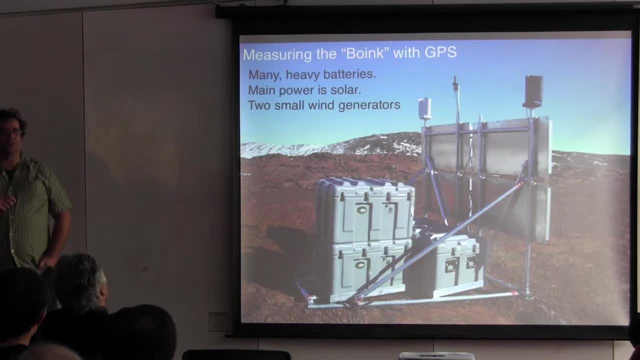 Four watts. Four watts doesn't sound like a lot. Four watts of power, Four watts of power. We're not going to bother with it, We're not going to put a regulator on it, because it's only four watts. Four watts can't do any damage to a battery system like this, can it? Four watts if you have 100-mile-an-hour winds on one blows your system to pieces And we've come back to find bits of other things that have come into point, which has spread over the landscape, So we now have regulators on those. 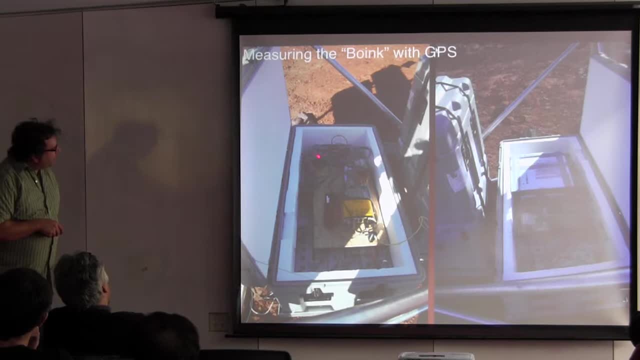 And they seem to work okay. Good, Here's some of the big batteries. We're using this really high-tech aerogel nanofoam insulation- the JPL design- And then someone decided that they would just slice off bits of the styrofoam. that you put in your home insulation instead. So instead of having $40,000 boxes, these boxes are about $1,000 each and the styrofoam is only a few cents, And that keeps the systems warm enough to run even through the coldest winters. 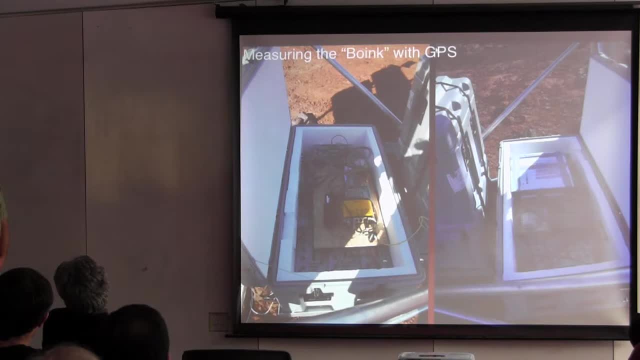 We've had these run down to minus 70 degrees Celsius. They've ran without a problem, Just lots and lots of them. We have a GPS receiver here, And then this is a satellite modem. So, as I said, we can look up these things. 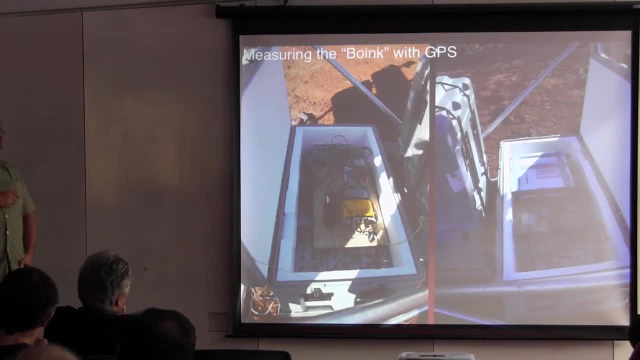 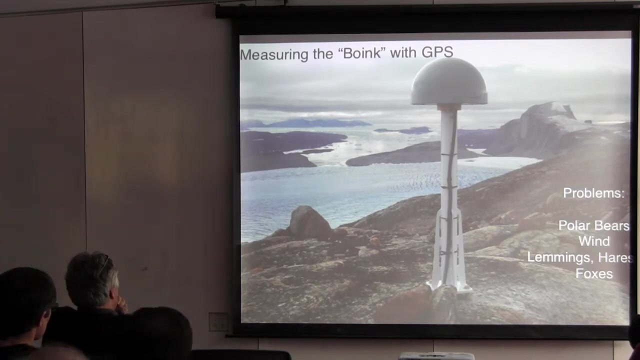 They broadcast in real time. If you go to the polnetorg page or the NAFCO page, you can have a look at the data that's coming off these with a one-day delay. Beautiful places, Problems- not so much in Antarctica. 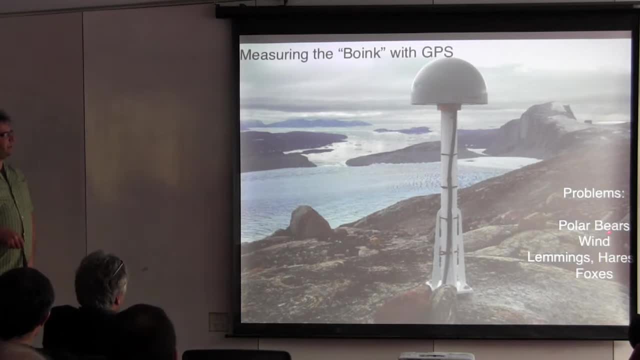 Problems in Antarctica have been due to static, but problems in Greenland have been a little bit unique. These things stand about seven or eight feet tall. We have little antennas way up here and we come back to find tooth marks where the bear has been on its side. 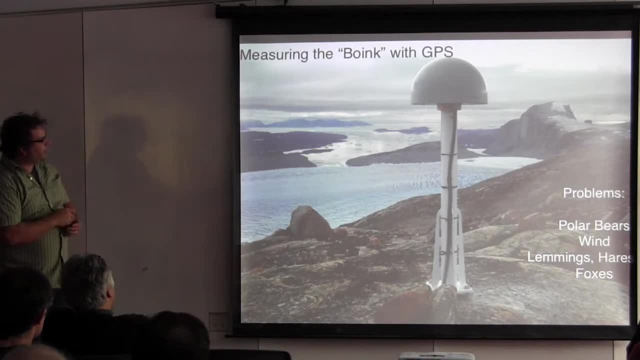 biting on them. These things are drilled about two feet into bedrock with four really hefty bedrock pins. So you want that antenna to be really strong. You want it to be stable When it's going up. you want it to tell you the landscape is going up. 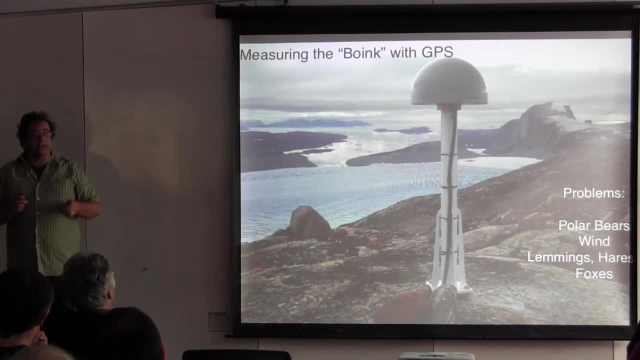 When it's going sideways, you want it to tell you the landscape is going sideways. What you don't want it to tell you is that a polar bear goes. this is a nice scratching post. That's them Some. where we come in. they've just been destroyed. 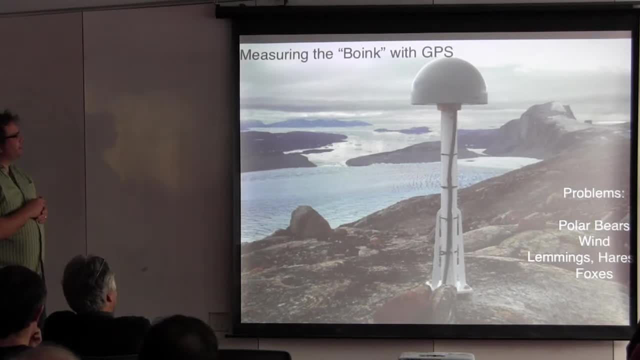 Wind we've had. These are decently thick pieces of plastic. It looks as though somebody shot them. It's not been, It's just the wind picking up rocks and throwing them through the air. We had one site installed in Antarctica where the team who was at the same place a year later 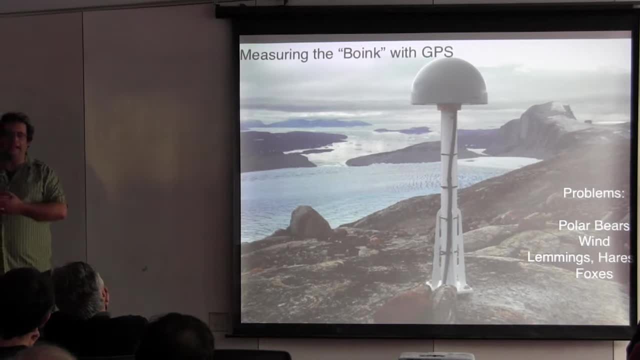 came out of their tent to see snowmobiles flying away at head height due to the wind. So the wind picks things up and throws them around in polar regions. The embarrassing one is we've had lemmings, and hares have decided to destroy our systems. 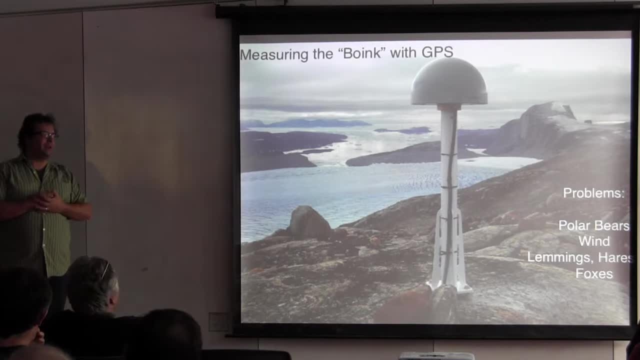 They found that they could chew through the electric cables. You've got 26 fully charged deep cell batteries. behind that We find bits of lemmings and bits of hair in the neighborhood. Nice and crispy. It spells Well. see, this one actually did. This one got beaten up by a polar bear And this one's about 2,500 feet above sea level And we thought we're at the top of these cliffs. Nothing's going to come up here and hassle them, Unfortunately. female polar bears once they've had their cubs. 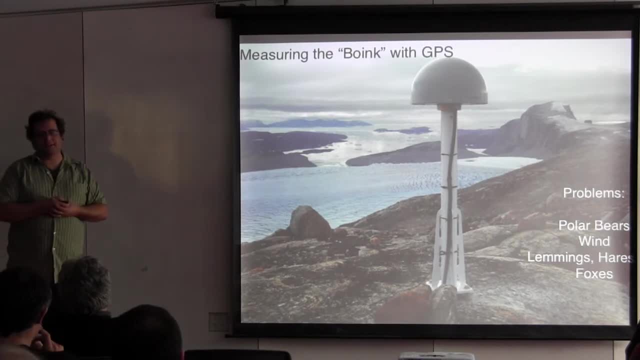 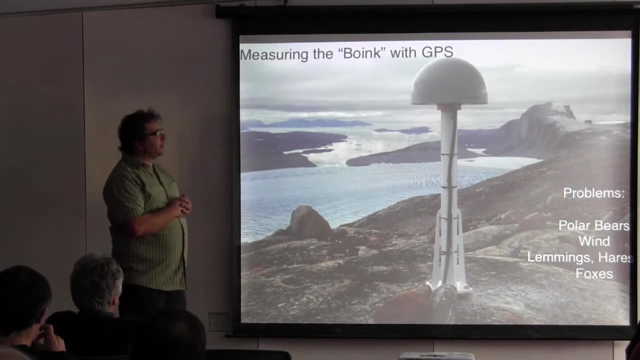 in the spring don't go anywhere near the sea ice, because that's where the males are And the males eat cubs. So the females come up to high altitude, crossing over really crevasse glaciers, And this thing probably smells like bacon to them. In the high Arctic there's not many smells, So to smell this they're just like what's that And they go and have a good nice investigation which causes us $60,000 to $70,000 worth of damage. 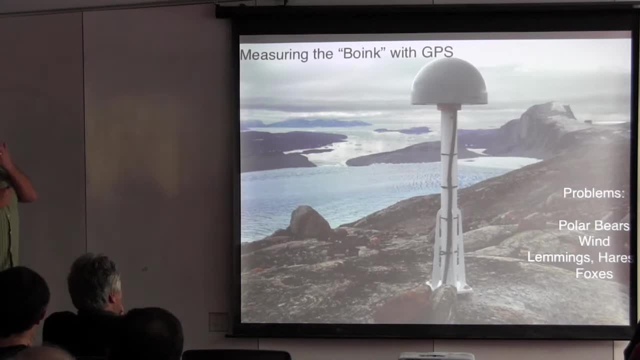 So we have to go and fix it And we have Danish colleagues who are like we can just polar bear-proof them And we're like: well, what does that involve? Well, you put a fence out And it's got barbed wire and razor wire. 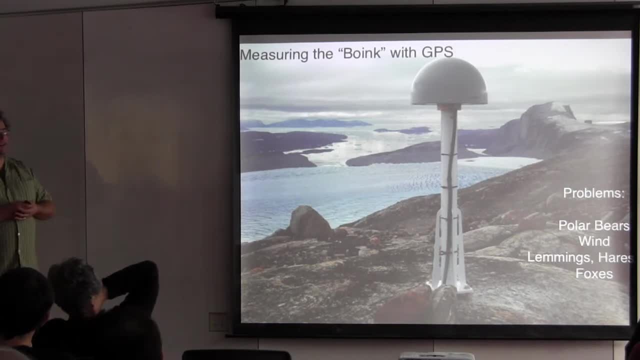 And it's got bangers and smashers. And we're like: and how heavy is that? Oh, it'll be, you know, 700 or 800 pounds worth of gear. And we're like: and how much is a helicopter to carry 700 or 800 pounds of gear? 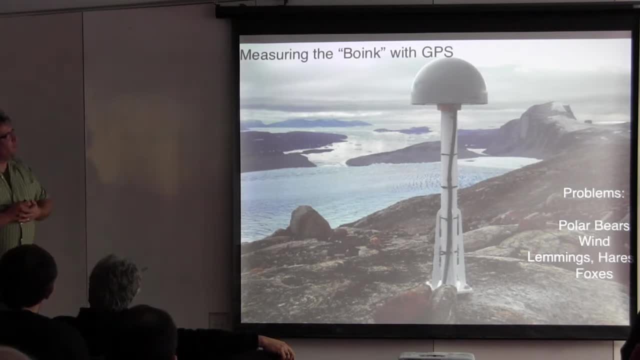 And it just ends up that we put them out and cross our fingers And we can. like I said, we lost three or four of them, But out of 55, that's not a bad going One site. we're eminently opposed to them putting it back in again. 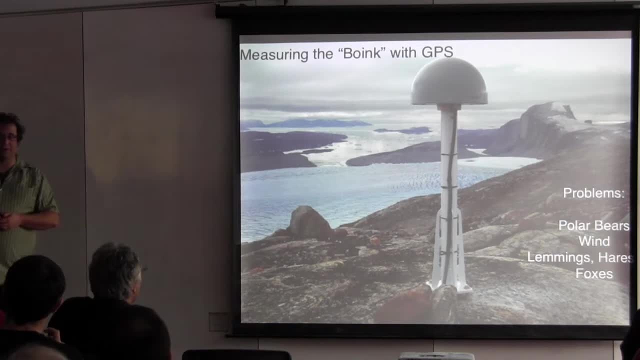 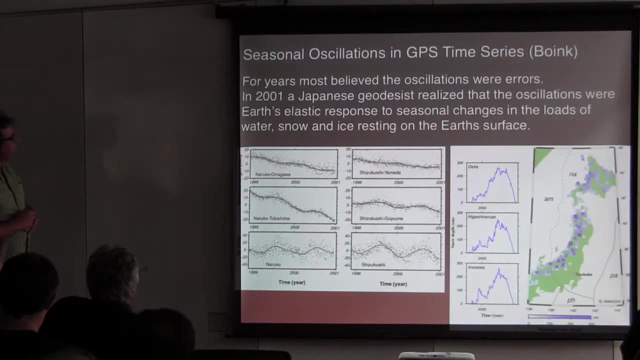 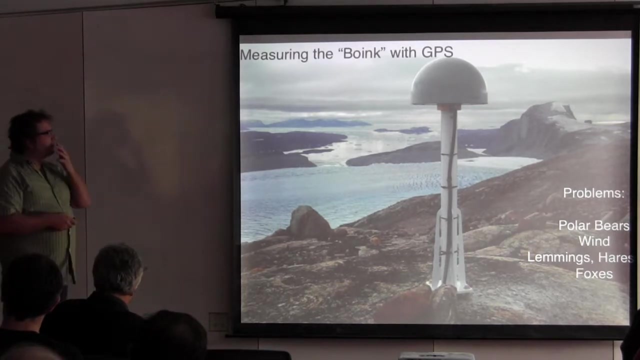 They keep on replacing it in the same place, But the bear obviously knows it's there. That was the scratching post one. But oh well, So these GPS, we get time series of east-west motion and time series of up-down motion through time. 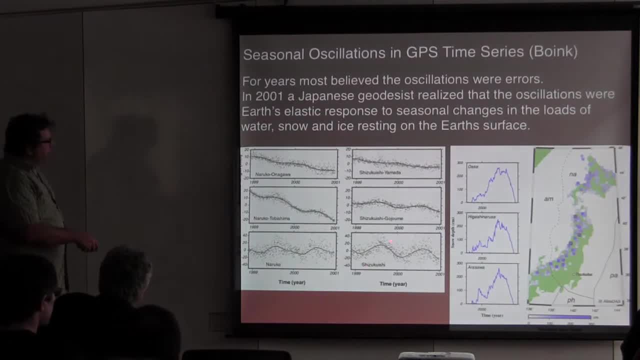 And they often make these kind of sinusoids. And for the longest time doing geodesy I mean, I started doing geodesy in 97,, 96, 97. And for the longest time we're like this stuff's noise. 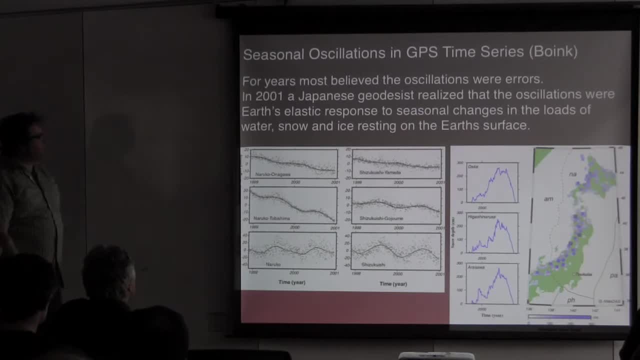 It's getting in the way It's bugging us. We have to just remove it. It's not telling us anything. In 2001, there was a Japanese geodesist called Heike who he started looking at how these things are bouncing in the air. 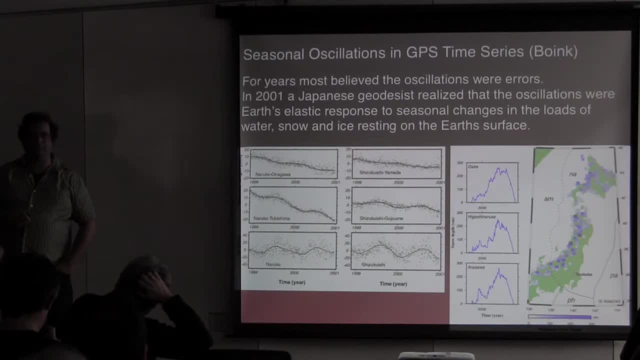 And looking at the local snow loads in western Japan And he found a one-to-one correlation: Snow falling next to this system, the system went down. Snow melting next to the system, the system went up. And it became clear that these oscillations. 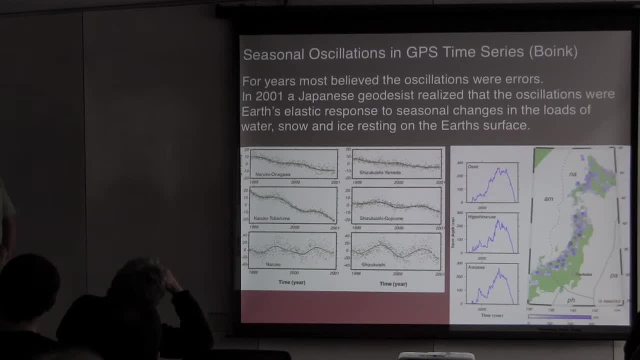 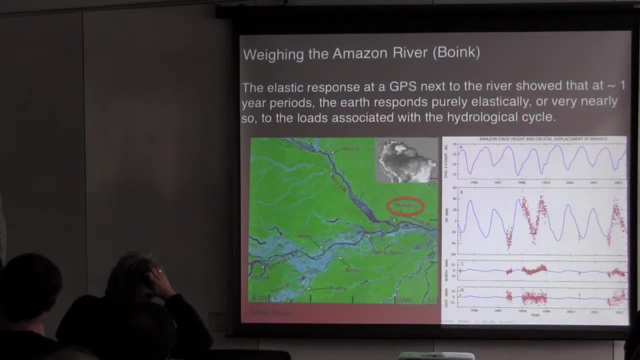 are at least partly caused by local loads changing around GPS systems. This is Mike Bemis, who I work with still on these projects, especially in Greenland. We have a GPS system at Manaus in the central, the Amazon basin in South America. 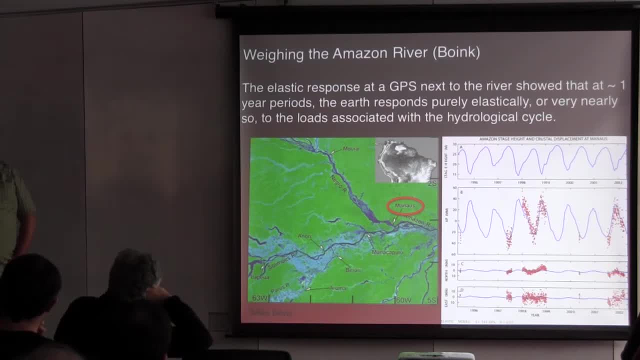 And there's a big flood wave that comes down the Amazon big tidal or reverse tidal bore. I guess that water comes from this direction, where the stage of the river goes up about 12 meters very, very quickly. And as the water goes up, the GPS goes down. 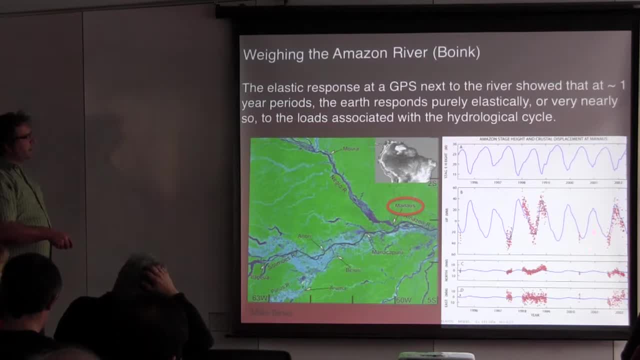 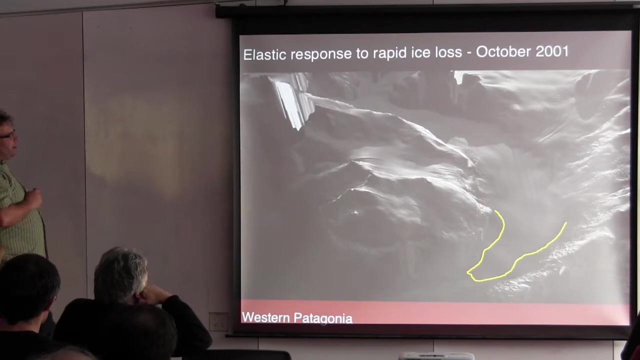 As the water goes down, the GPS goes up And he showed pretty convincingly that you can measure these elastic deformations due to hydrology, at least in this part of South America. So glaciers do they give you elastic responses? This is a glacier. that's kind of hard to see in this light, unfortunately. 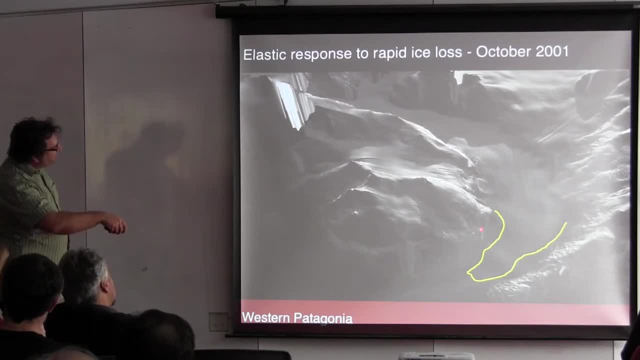 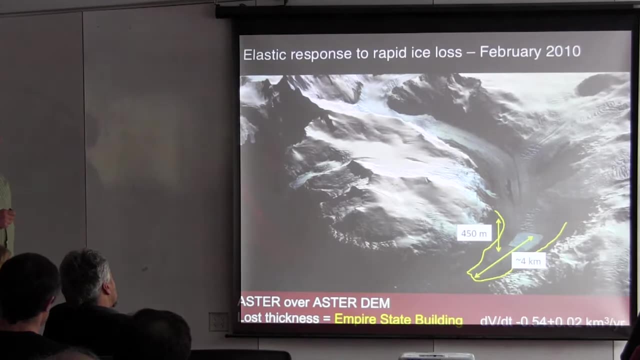 It flows down here, down here, And this is where the front of the glacier was in 2001.. This is in western southern Patagonia. This is nine years later, in February 2010.. And there's the outline where the glacier was. 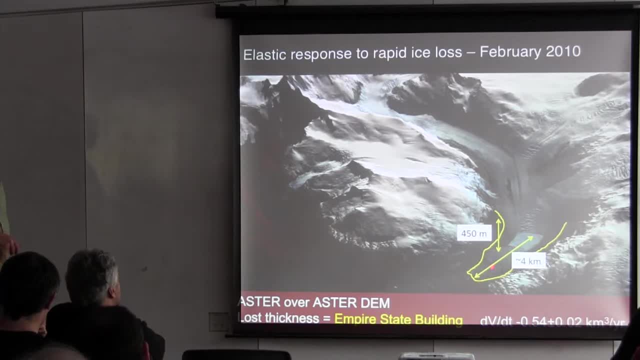 And here's the front of the glacier now. So it's gone mad. It's four kilometers of ice has been destroyed And the vertical is 450 meters of ice difference. Empire State Building is 458 meters tall, So in nine years it lost the thickness. 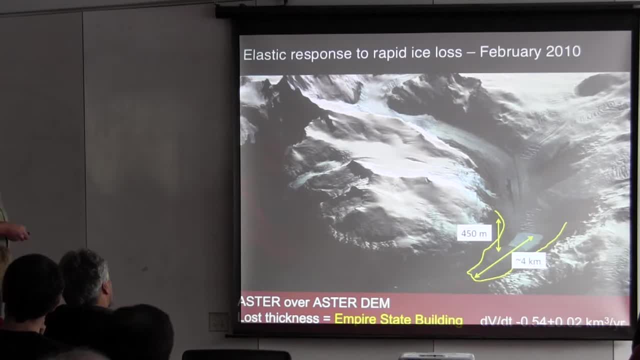 of the Empire State Building. at that point You can be very, very sure that the bedrock next to this is springing up in response to that And we will try and get again this summer to get funded to go and put GPS in it to measure that. 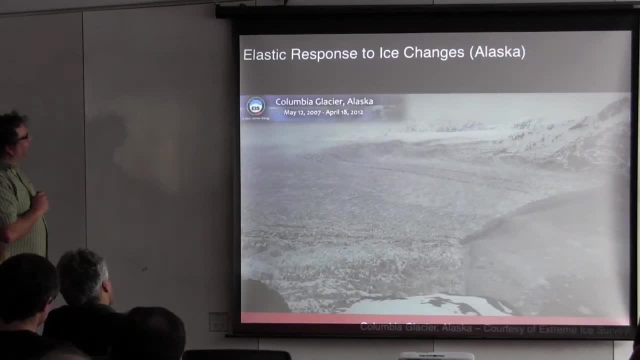 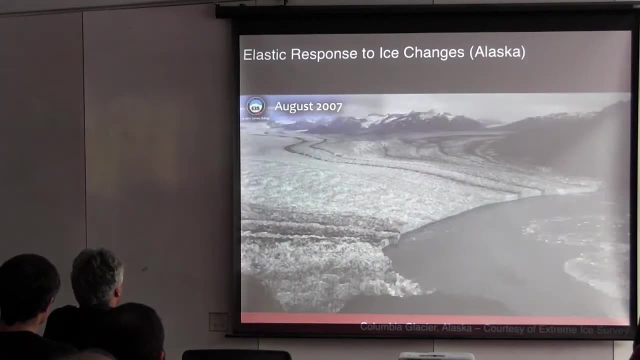 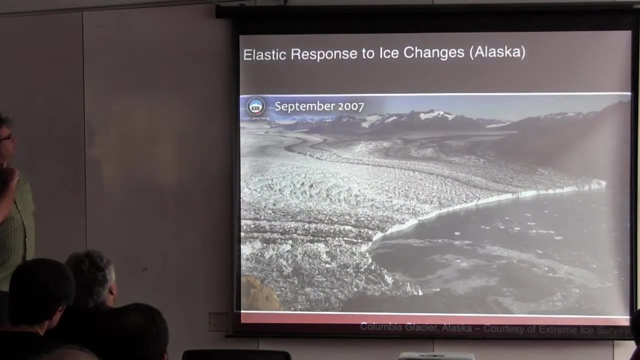 We're not back on that proposal whatsoever yet. So just, is this going to work? Yes, So this is the Columbia Glacier between 2006 and, I think, 2012? 2010. maybe From the Extreme Ice Survey, which is a, you might have seen Chasing Ice. 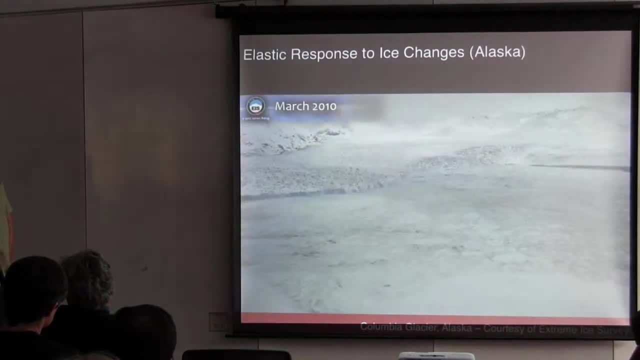 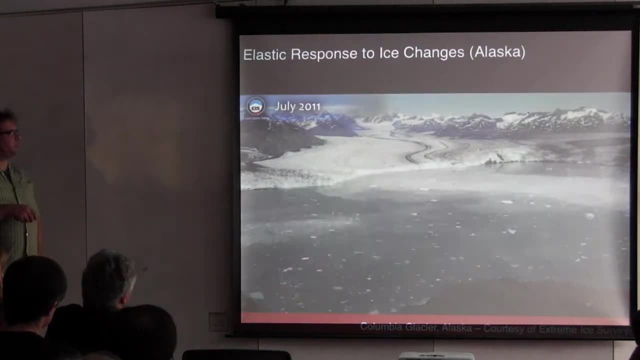 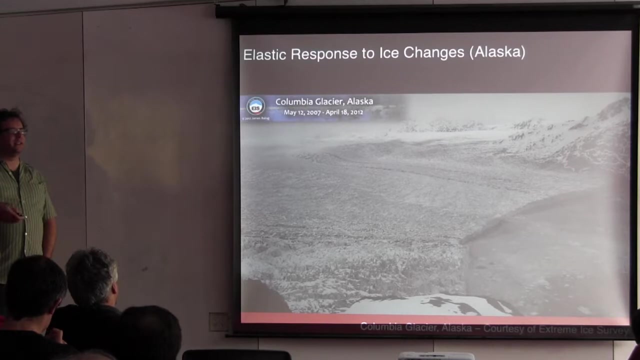 It was the film that James Balog put together using this sort of footage, And so the glacier going back like this isn't the biggest signal, because, as the glacier goes back, you can see the water fills in where the glacier was, So, in terms of a mass, 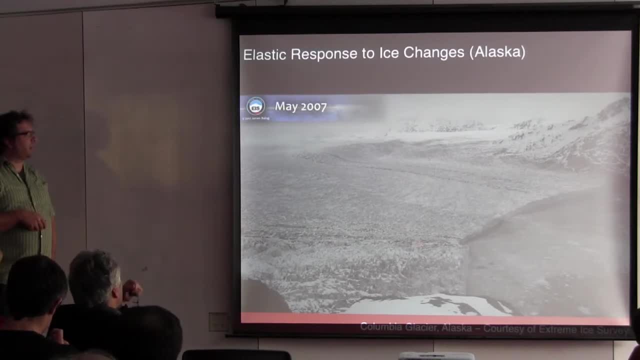 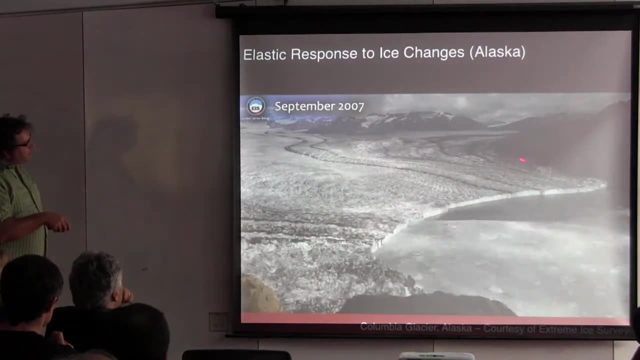 that's not really important. This glacier is probably floating already. It's not really at its sea level. What we're more interested in is these trim lines along the edges of the glacier where this ice was sitting on the earth and now it's going into the ocean. 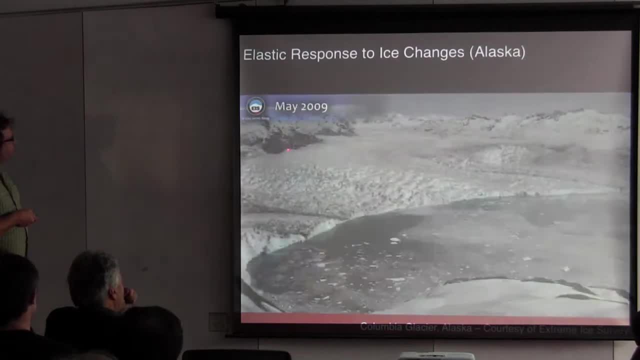 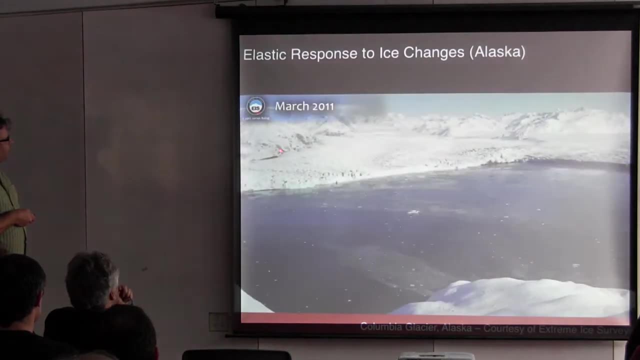 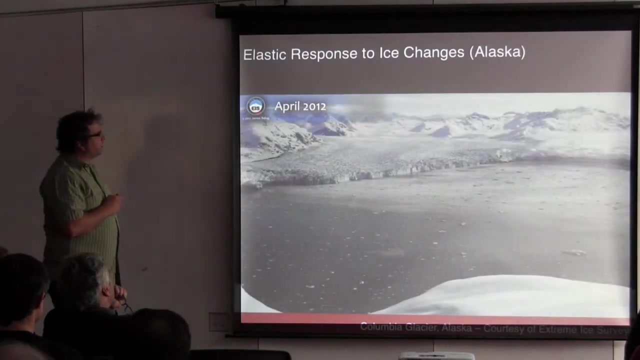 It's got a lot of them And that's it, Kind of watch it deflating there My cursor is, or my pointer is, where the edge of the ice used to be, And that's probably several tens of meters, which is the sort of signal that the GPS will pick up. 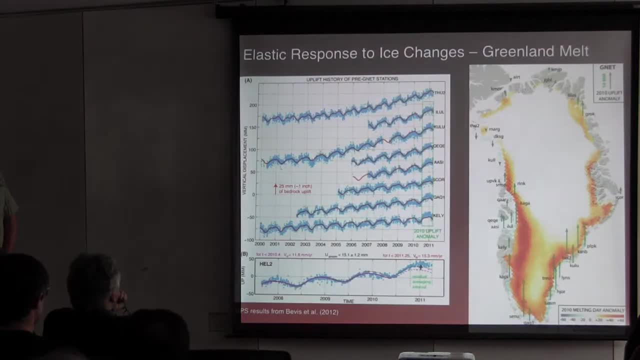 as an elastic response very easily. Okay, this is a brain bender of a diagram. The site that gets eaten by polar bears is here. The other site that gets eaten by polar bears is here. so there's no arrows for those ones, strangely enough. 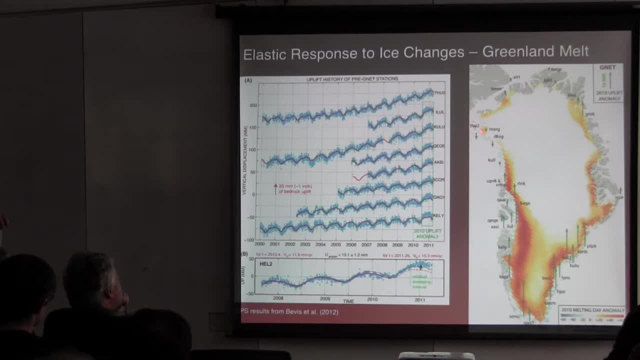 What we found in Greenland, and this is: let's have a look at Thule 2.. Here's Thule 2.. What we found in Greenland is: this is what the ice used to do. This is what the GPS did. This is what GPS used to do. 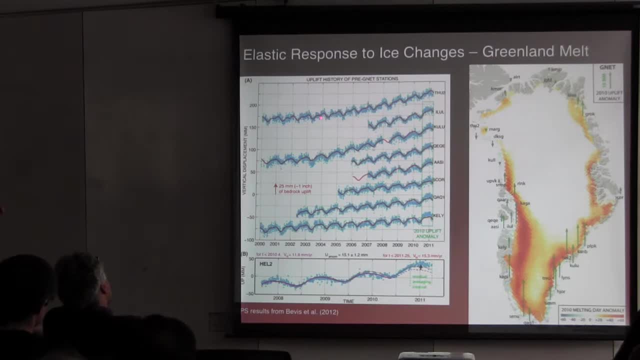 It was kind of doing nothing, just annual cycle, And then about 2003,, 2004, it started getting a bit faster, and 2006,, 2007, it started going a bit faster still. So there's a bend to this trajectory. 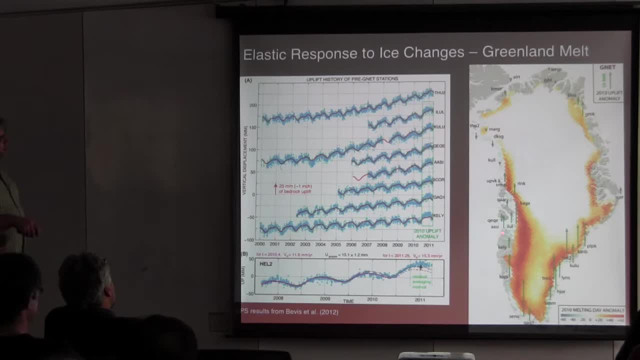 that you wouldn't expect if it's going on faster. Elulissat down here. I'll show a longer time series for that. in a second It's doing the same Colosso down here. it's going on faster. 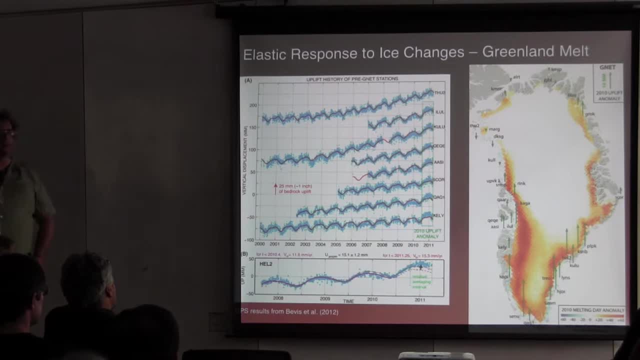 A lot of these sites are going on faster, Faster than they used to do- And we actually can take this back down to, almost, in fact, a yearly level and say: if we know what the long-term behavior of these sites are, we can predict where it is through the year. 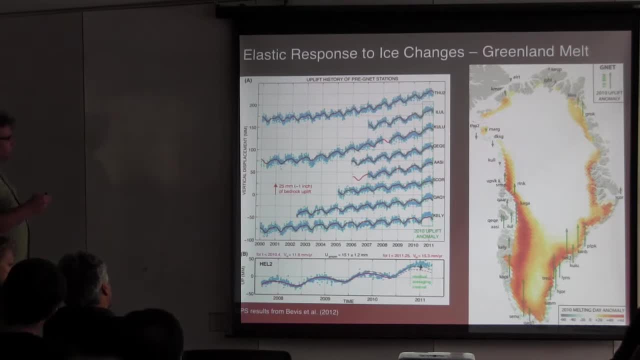 and then we can have a look at the difference with where it is compared to the average, And what we're showing here is this is a map of what's called the melt data anomaly for 2010 in Greenland, So where it's very, very red. it melted 60 days longer than the 30-year average in 2010.. And you can see that the GPS at those sites are springing up. Where it didn't melt any longer than usual or just slipped longer than usual, the GPS isn't doing anything. 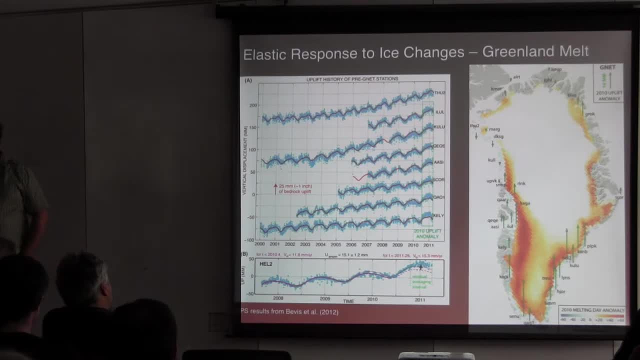 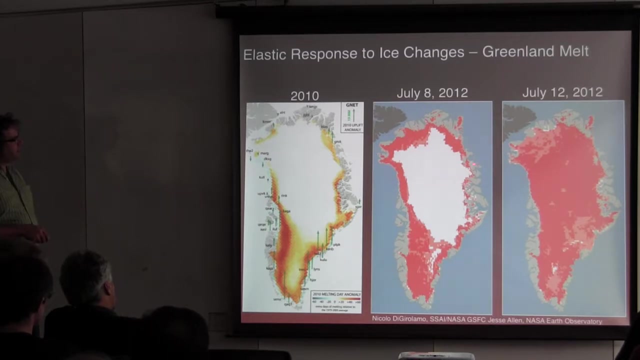 So we're really pretty accurately being able to measure what the melt is doing in 2010.. The data in Greenland: the surface mass balance with the GPS And this was 2010.. So this is 2010. over here, This was July 2012, or July 8th. 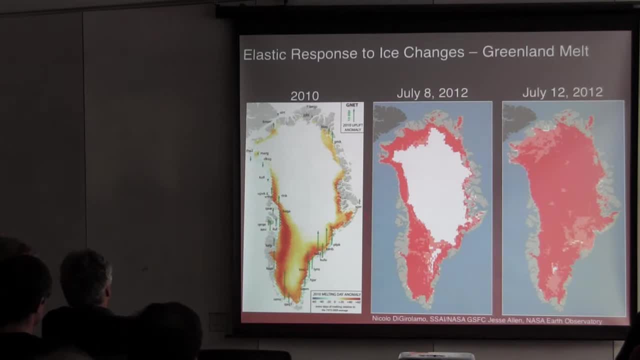 And this is four days later, And these are pixels of melt And we've not seen this before. 2013 was nowhere near this sort of coverage of melt, But basically in 2012,, the entire of Greenland at some point. 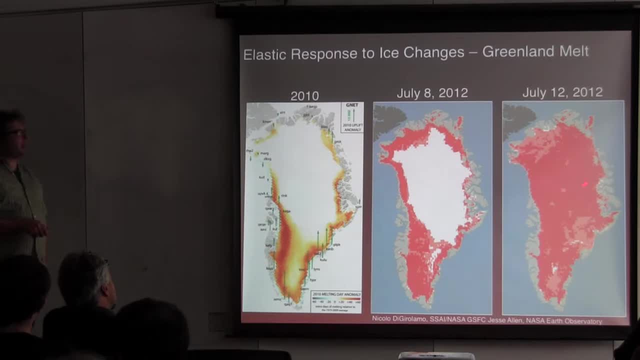 melted, Which even up to the highest elevations you know, 3,000 meters above zero. 2013,- this was a lot smaller- 2014,. put my neck out here. I expect it to be kind of 2012-ish. 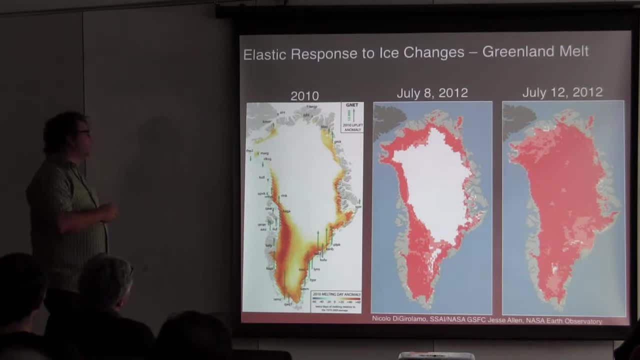 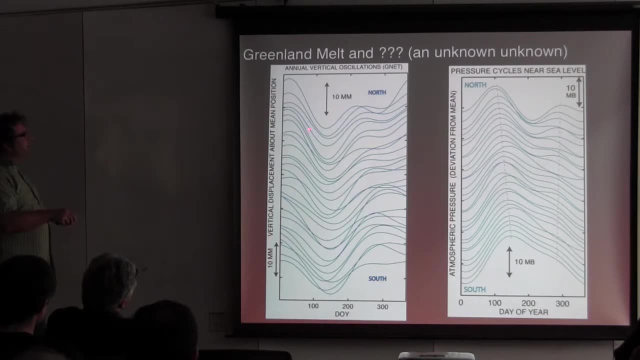 based on what we've seen already in the last two months, Although that could change. So we're getting all these bounces in the GPS signal, So this is each station. This is what they do on average per year And we looked at that. 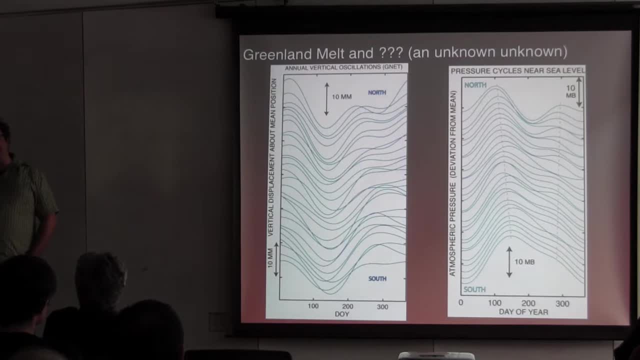 and then we looked at GRACE, And GRACE gives an independent measure. So this is what the bedrock's doing in the up. We looked at GRACE and GRACE was telling us this is what the mass changes are, And they didn't match. 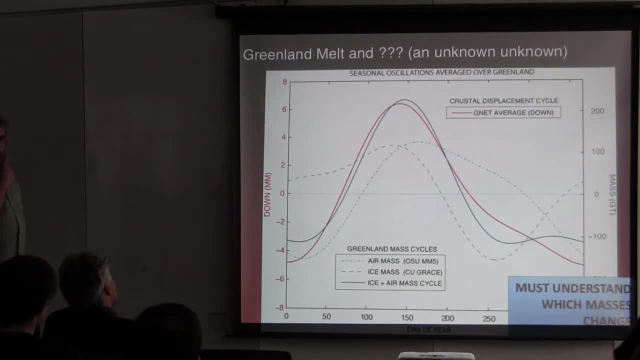 They were shifted in phase. So we got this blue line- pardon me, we got this red line for what, on average, a GPS site in the edge of Greenwood does each year. And then we looked at GRACE and we just we said 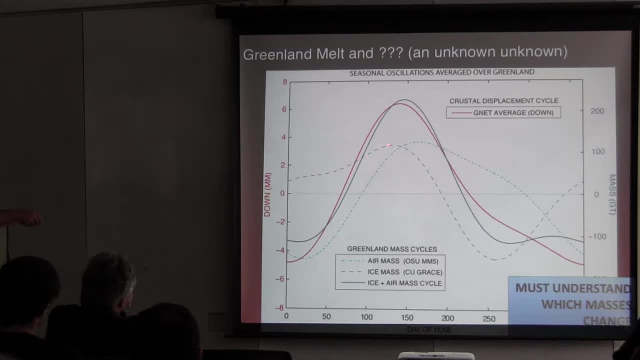 okay, what does GRACE do? GRACE has this big dotted line here and you can see it doesn't really match the red line. Mike and I sat and talked about this for a very long time And we came up with this dotted line. 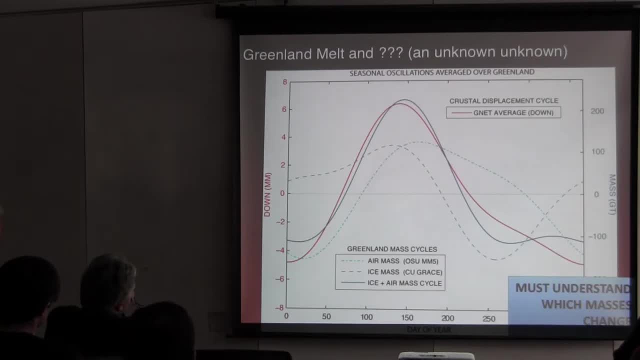 This dotted line is the weather systems On average for Greenland throughout the year And we added the two together and we got the blue line. And what that's telling us is the GPS are measuring the mass change caused by changes in ice. 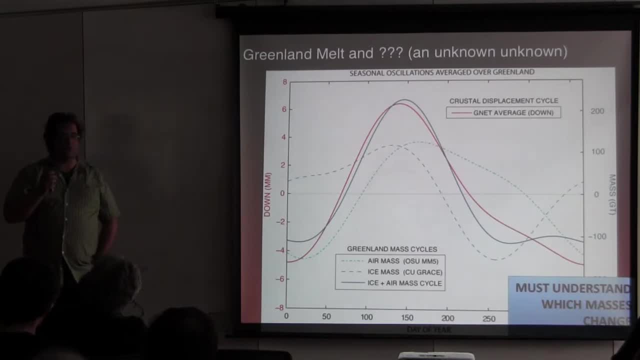 in ice melting and the mass change caused by the average weather at the GPS site. So as the high pressure system comes over the GPS sinks, As the low pressure system comes over the GPS rises. So we're actually measuring weather with by measuring the elastic response. 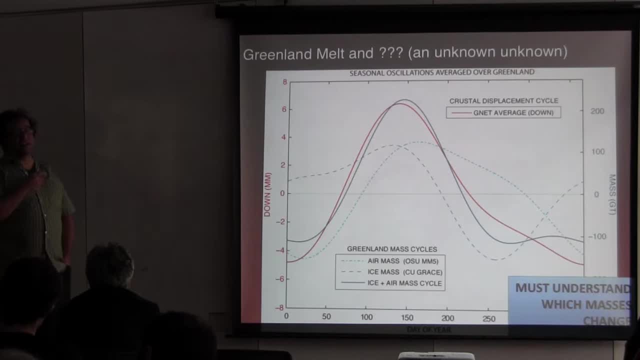 of the surface of the Earth, which that was an unknown, unknown. This was a surprise to us that we built this. And this is not big numbers. These are what: six, So this is 10 millimeters, So a centimeter, half an inch. 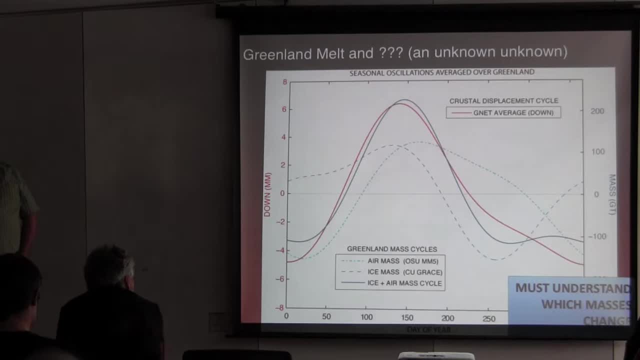 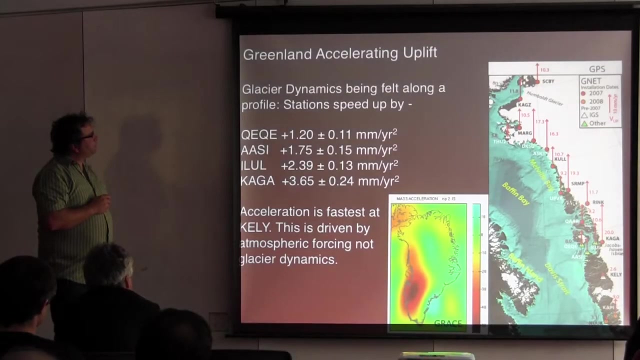 But there's a half inch oscillation on average at a GPS site in Greenland, caused by ice mass changes plus the weather, which we need to understand- both of those- in order to back out all these long-term signals. So I'm just going to go a little tour. 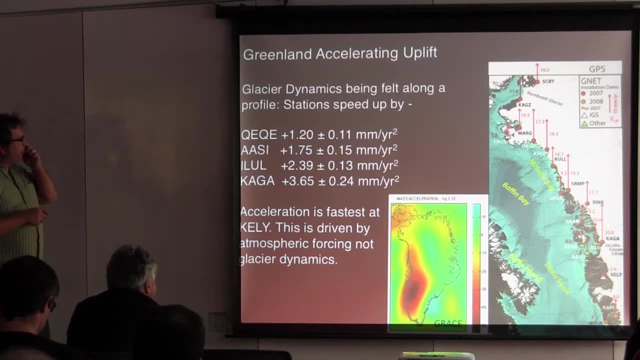 around bits of Greenland And what we found. so there's four stations here. I'm not even going to pronounce it, because I can't pronounce it. That's the Danish name: Asiat, Alulisat and Kaga is effectively Jakobshavn. 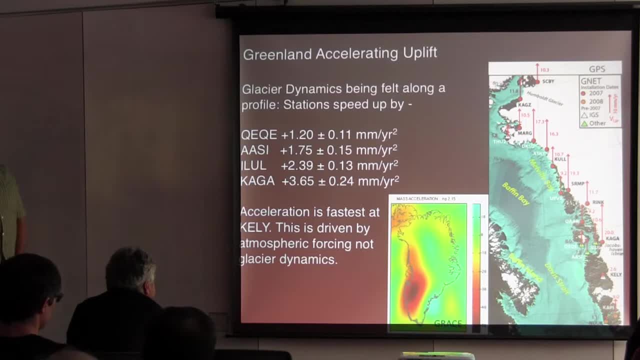 which is the glacier which they say sank Titanic is the glacier that's been in the news recently for just going super, super fast. So if we take a profile along those GPS sites we get the site that's on the coast there over the last, you know, six or seven years. 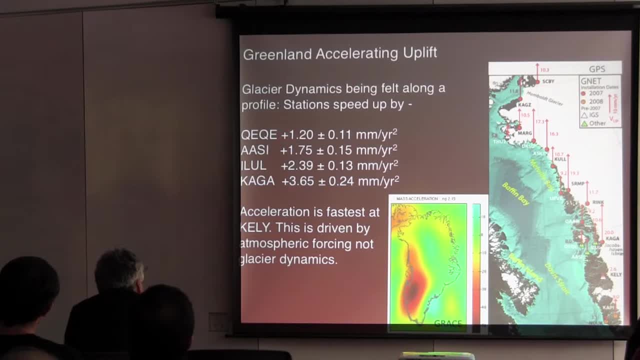 each year has been going up faster. So in year one it say was zero, Then year two it was going up 1.2 millimeters per year. In year three it was going up 2.4 millimeters per year. 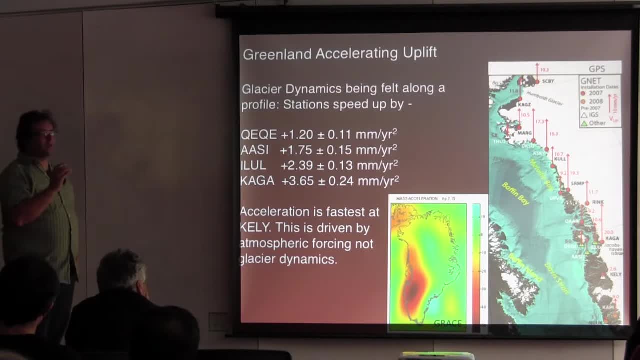 In year three it was going up 3.6 millimeters per year. In year four it was going up 4.8 millimeters per year. So it's accelerating at 1.2 millimeters per year. upwards Asiat a little closer. 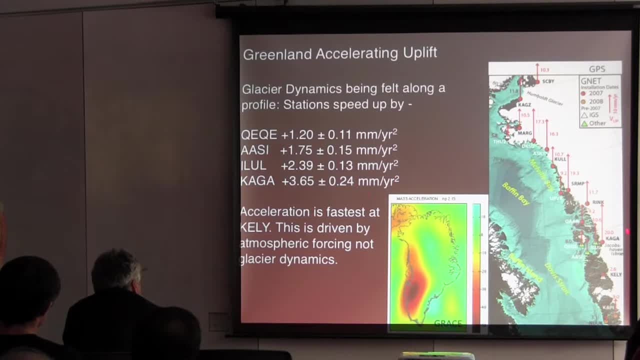 1.75 millimeters per year, Alulisat almost 2.4 millimeters per year, And the site which is right next to the calving front, where the thinning is occurring, is going up 3.6 millimeters per year. 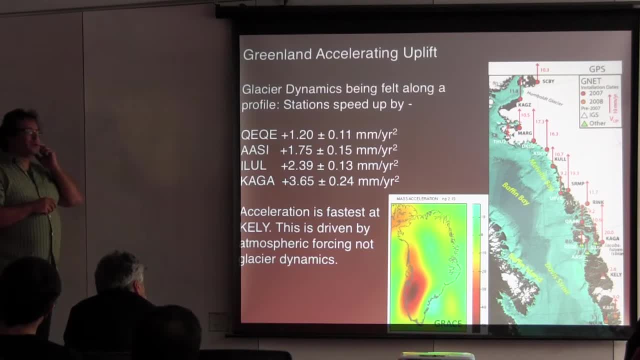 faster every year. So this is just a constant acceleration that's occurring and that's due to the mass loss that's occurring as Jakobshaven gets faster and faster, and faster, and thinner, and thinner, and thinner, Actually, in all of our GPS sites. 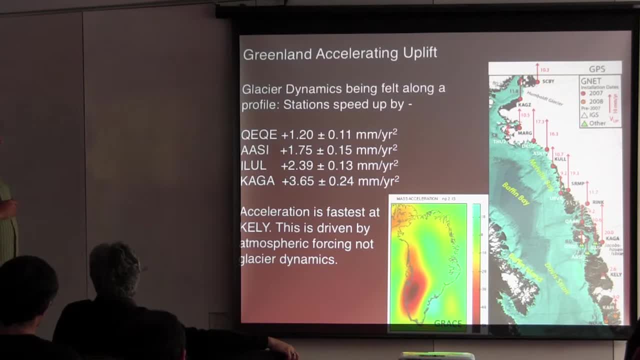 around Greenland. there's a rather unsupposing one down here in Kellyville, which is where the main American research takes place- is going up at an accelerated rate- faster than anything else, because when we first started these surveys that was going down. 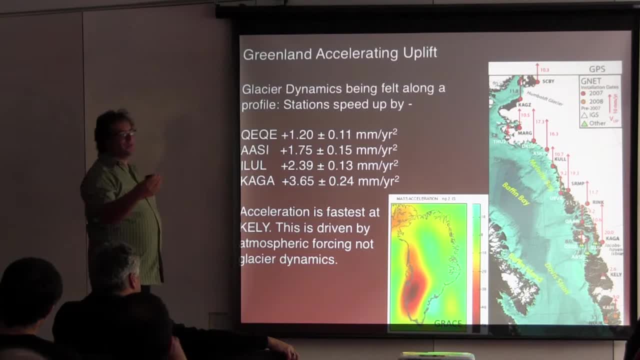 So the system there was going down through time and as we get closer and closer to present, it's now swapped its direction and it's now going up 2.5 millimeters per year, And that's actually fairly gratifying, because this is GRACE. 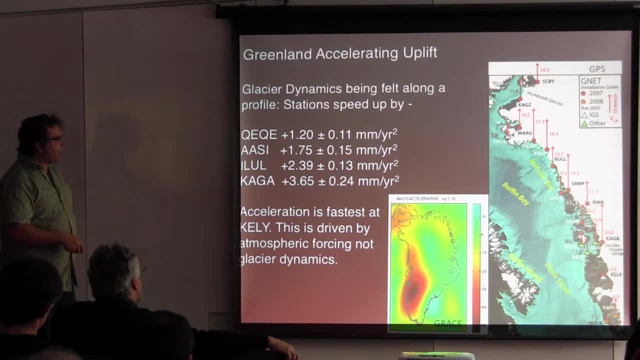 This is the GRACE map from 2003 through 2010 of accelerations, and you can see this bullseye of faster acceleration going on in the southwest, which is nice. The thing with Kellyville is there's no glaciers that go into the oceans there. 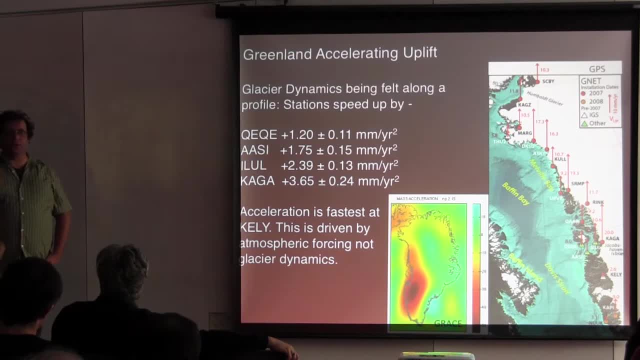 All the glaciers end up on the land, So you can't have glaciers going faster at Kellyville to give you the ice changes. So all the changes that are going on in Kellyville are purely due to accelerated melting or a change in the amount of ice. 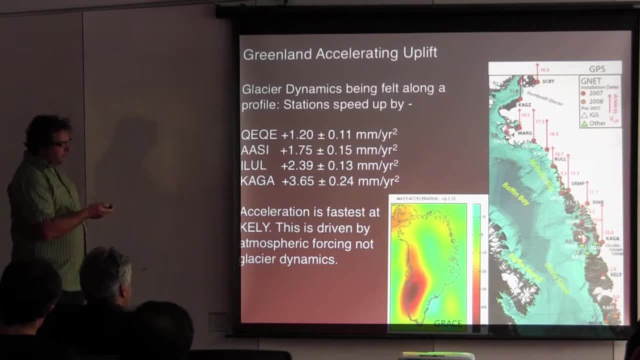 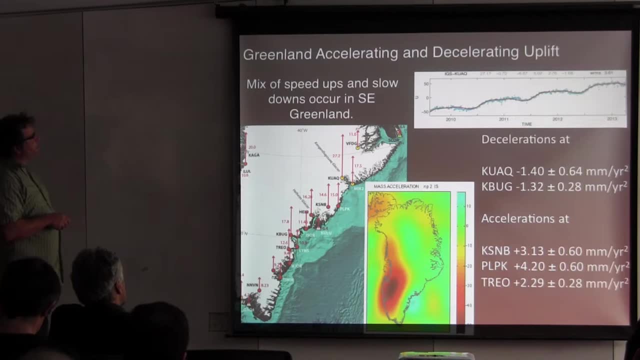 that's falling year after year after year Again. this is just an example of the sort of time series that we get from the GPS And down here in the southeast, which is my personal, probably my favorite place on the planet. it's just gorgeous there. 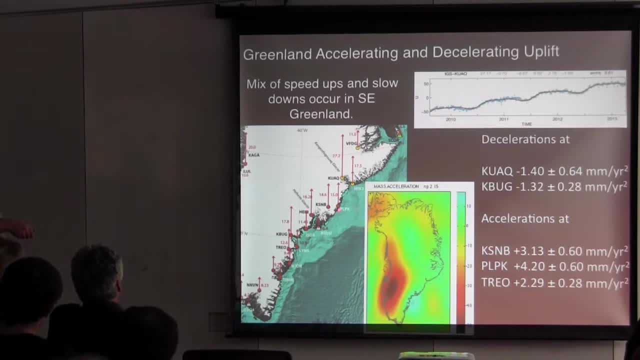 less polar bears, which is good. This one got eaten by the polar bears, so I'm completely free. In southeast Greenland we get a mix. We've got sites that are going down. This one up here: Kua and Kangu Shua Glacier. 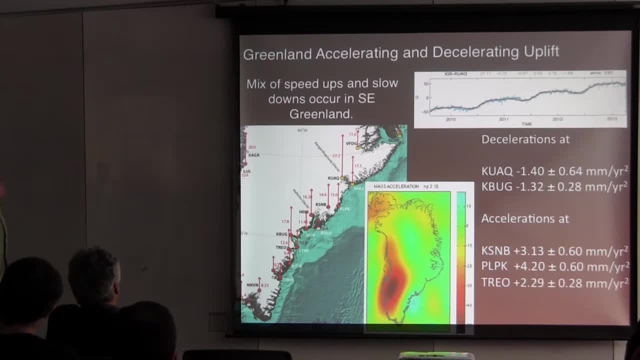 and this site down here in Kebab. They're going down year after year at a faster and faster rate, Whereas, mixed in with those, we've got sites which are going up pretty quickly year after year after year, And you can see Grace here. 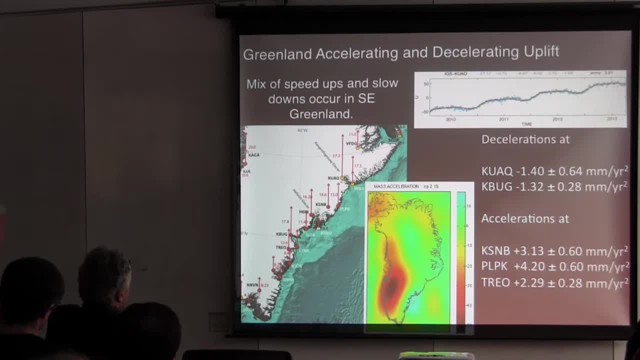 just says that everything should be slowing down. And that's just this. This was another unknown. unknown. Grace says that you should have just slowing down glaciers in southeast Greenland. But we've definitely got. we've got some glaciers slowing down and some glaciers speeding up. 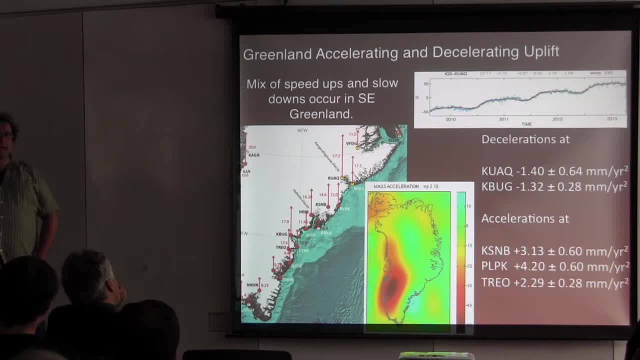 And it's just the resolution. it's just the horizontal resolution of Grace. Everything over a 300 kilometer pixel smears out the fact that some glaciers here are shooting off into the ocean and some glaciers are doing nothing. So this is actually providing. 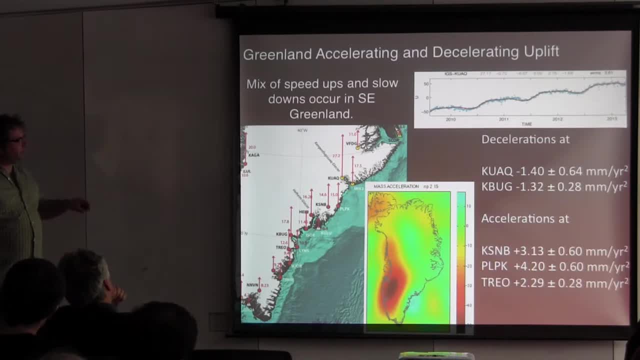 more information on top of Grace to say that on a basin level or on a glacier by glacier by glacier level, things are much more complicated than we thought, Which has led us to I'll take a bit of a step back, because Grace has been the benchmark. 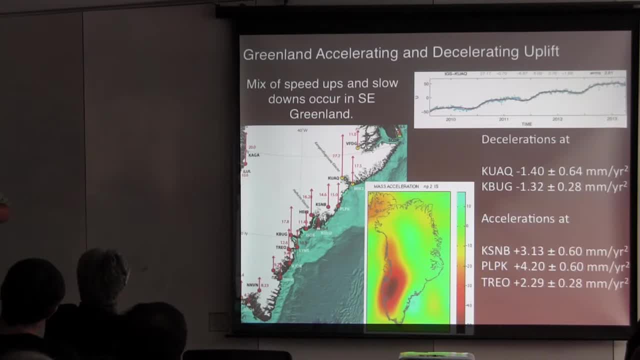 Grace has been. Grace is telling us what the Arctic, or Antarctic, is doing. This is saying Grace isn't telling us the full story And it is saying that if we're smart with where we put the GPS, and then if NASA and National Science Foundation 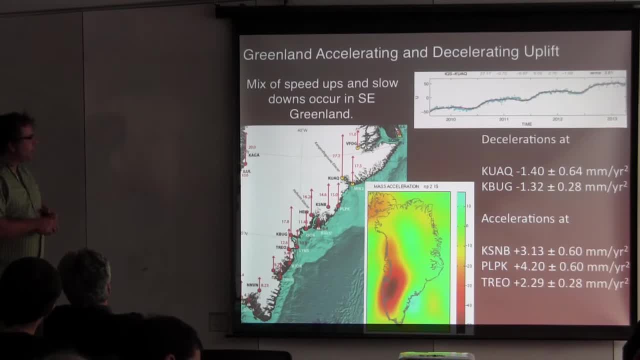 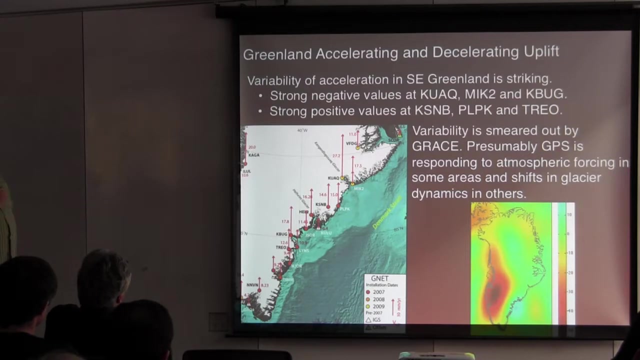 decide to keep paying for these things running. we can actually weigh the ice sheet in a matter that's complementary to Grace and lets us make even finer scale measurements of the mass changes. So the variability of acceleration in Southeast Britain is striking. We've got some sites going down. 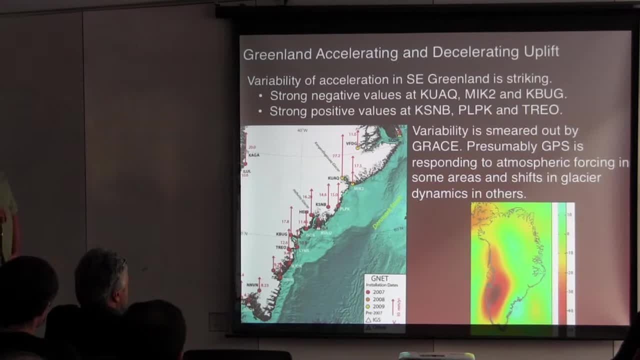 some sites going up and it's smeared out by Grace And some things are going to be caused by atmospheric changes. the amount of snow, the amount of ice and others are going to be caused by the changes in the speeds of the glacier. 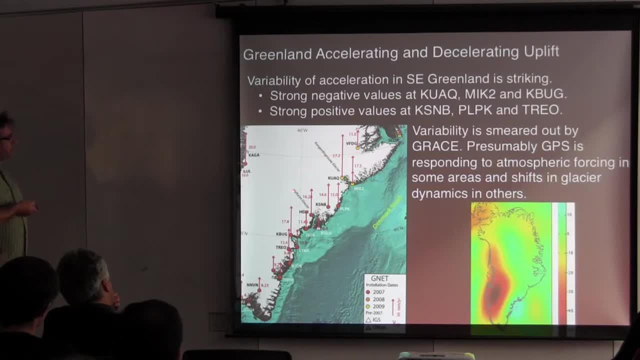 So this Camelot Shire Glacier is a really big glacier. Hellhound Glacier, a really big glacier. They were thought for the longest time to be the main methods that Greenland gets ice from the interior into the ocean. Jacobshaven was the other one. 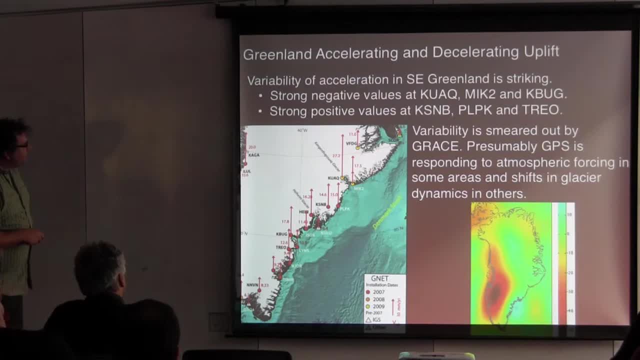 which is over here. I was at a meeting a couple of weeks ago that I was. I have to say this: I've always said that this little unassuming glacier down in Southeast Greenland is a monster, putting lots and lots of mass into the ocean. 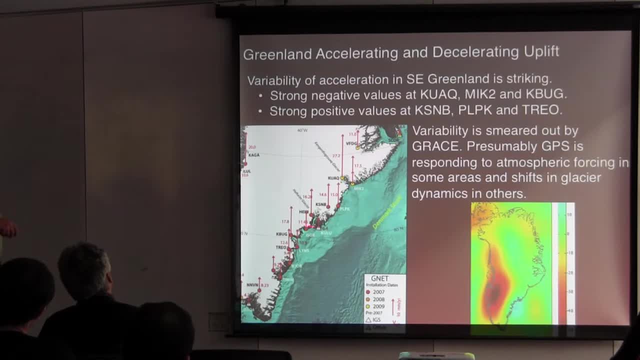 It's vindicated. It showed that, out of the big three, these ones are third and fourth, and this guy's second, in terms of mass throughput into the ocean. So this one's slowing and this one's slowing, but these ones around here are speeding still. 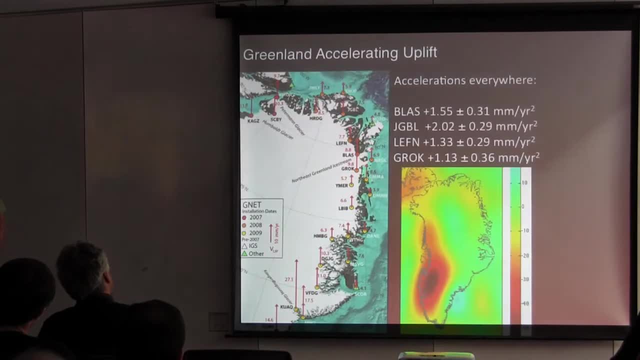 And Grace just can't show it. So going up to Northeast Greenland, basically everywhere's accelerating. All of them are getting faster year after year after year. This might be the next area where Grace sees that mass that came up to the west coast. 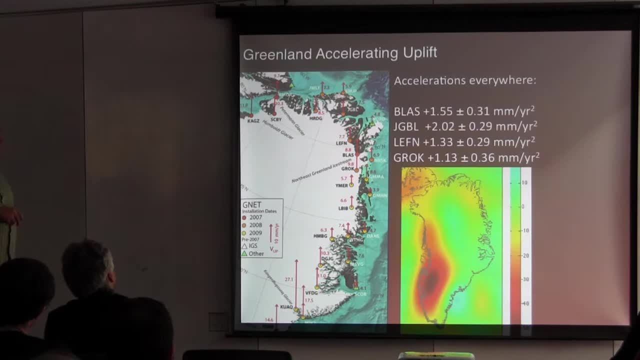 It's going to be going across the top, And this is a little bit interesting because this particular ice stream, most of its base, is below sea level, so it has the capability of shoving more ice into the ocean faster than we thought. I'm working with some colleagues up in Buffalo. 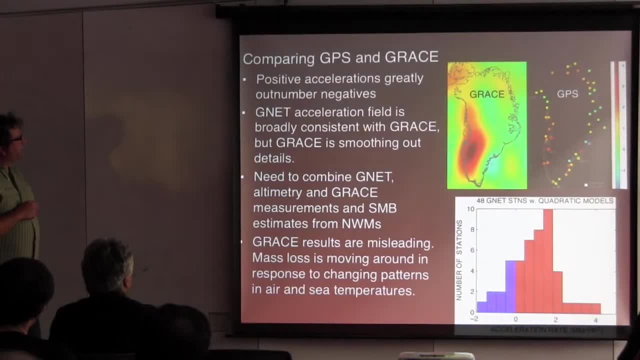 to look at that a little bit closer. So this map is probably the one we'll look at. This is the Grace acceleration, hot colors being things that are accelerating, blue being decelerating. Same color scale over here for the GPS and you can see the vast majority of the GPS. 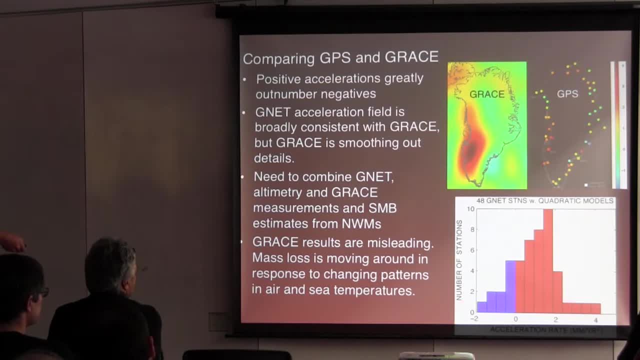 things are hot colors. So out of the 48 that we didn't have, polar bears eating them, you've got one, two, three, four, five- what's that? 10.. So 38 of the 48 stations are getting faster through time. 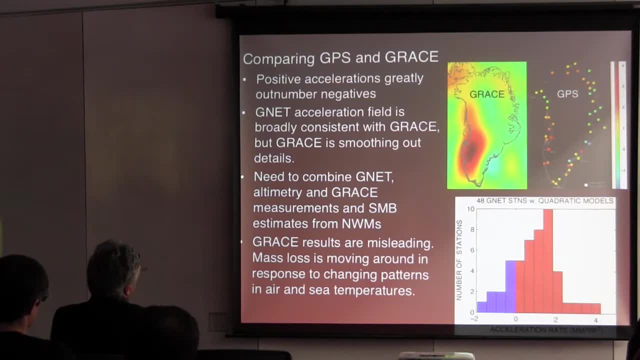 10 of them are getting slower through time. So Grace is a little misleading saying all the story in Greenland is going to be over. here We've got a mixed-in story just because we have slightly better resolution. So really we need to come up. 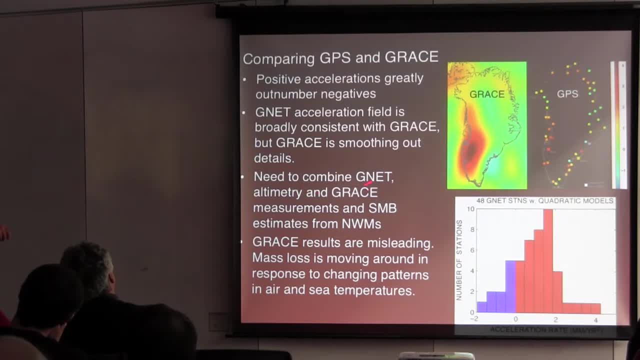 G-NET is our acronym for the GPS, the Greenland network. We need to combine the GPS with altimetry, with grades, with surface mass balance measurements and with results from numerical weather models to really get a handle on how much is dynamics, how much is snowfall. 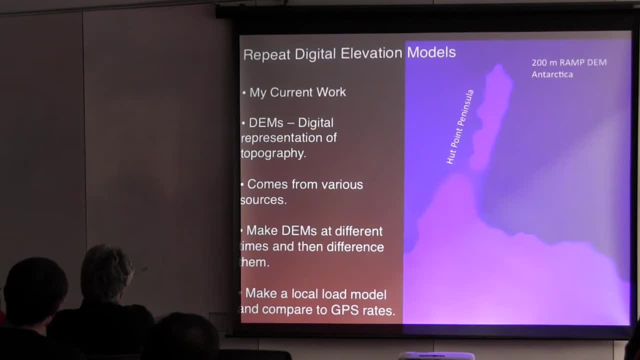 and what Greenland is doing to the sea level. So this is something that I've been doing while at Cornell and while at UNC, which is- I'm switching this now to- to Antarctica- at least one You've been to, McMurdo, is that right? 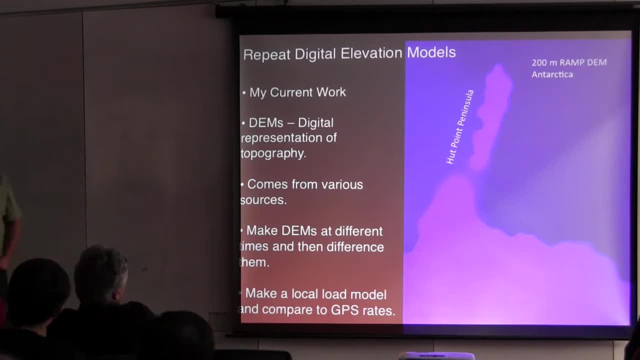 You said you were with the guard Or you've been with the airlift. Okay, So you just saw. you saw the jacket, you saw the boots. So in Antarctica, Ross Island, there's a peninsula that goes out in Ross Island. 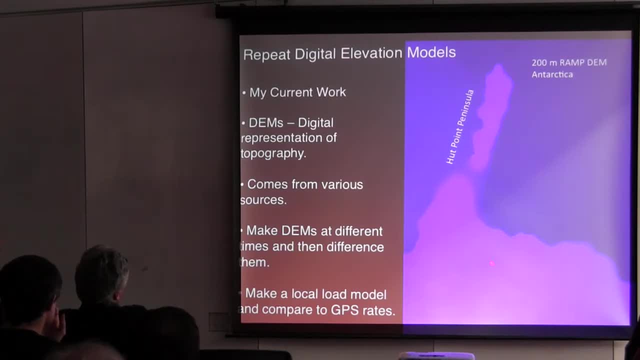 This is a volcano and it doesn't look like much in this, because this is the best digital elevation model that we had for the region up until about 10 to 12 years ago. So I'm going to be talking about DEMs. 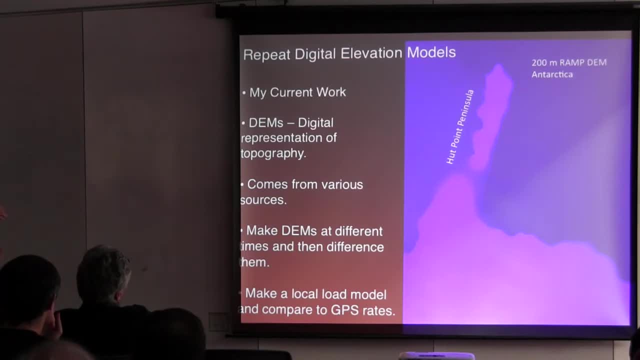 which is just a digital representation of topography and the various sources they come from. But if we get DEMs for the same place at different times, we can remove one from the other and have a look at what rock or ice is being doing. 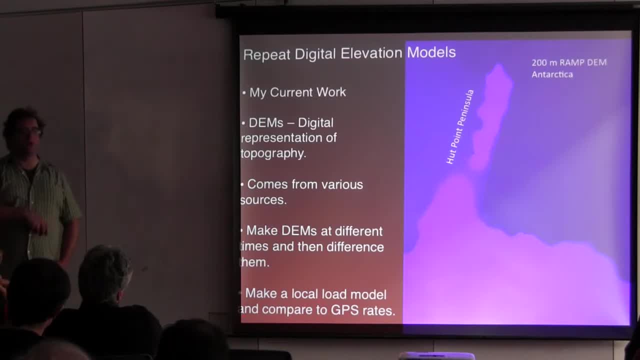 And then I'm making local load models which I'm going to throw at the GPS and try and get a handle on some of those annual variations. So this is a 200-meter resolution. it's called a RAMP DEM, Rigor-Sat-Project DEM. 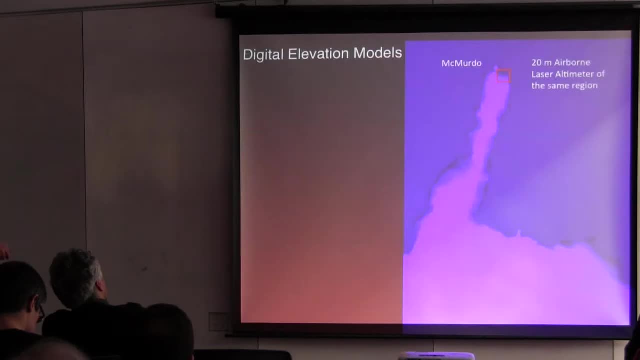 Then this is a 20, you see a little bit more information. you can see kind of a little peninsula coming out here. This is a 20-meter gridded DEM from a laser altimeter that they flew in 2001.. I'm going to eventually zoom in on the American base there. 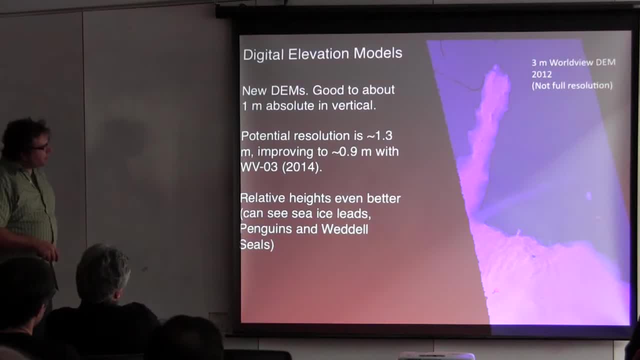 This is what I'm currently working with, which is a 3-meter DEM. You can see a lot more texture coming in. There's actually an ice tub there. It's kind of hard to see in this light, But we're making this with spy satellite imagery. 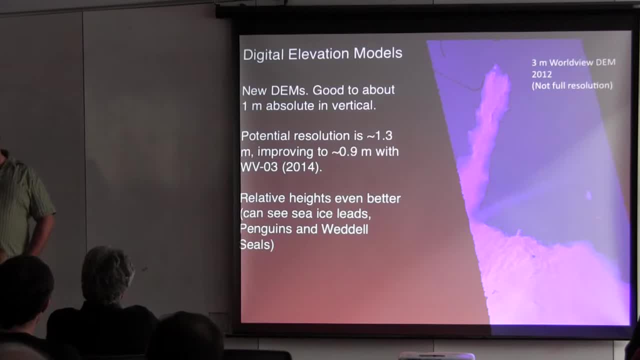 The federal government has arranged it so that people working for federal agencies- NASA, NSF- can get their hands on spy imagery And when they take two images with the same place, we can make a 3D model of the place. Potentially, 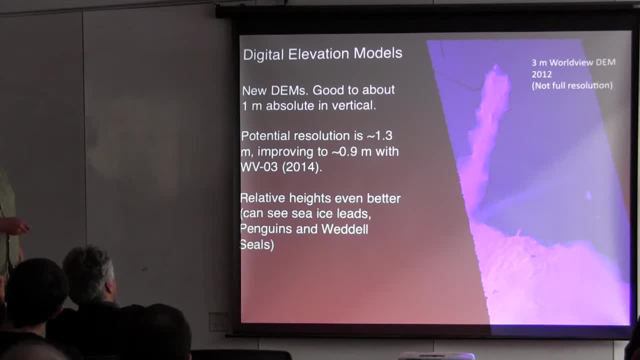 that can be as good as 1.3 feature postings. I'm doing three just now, just because it's easier to compute. There's a new satellite going up at the end of September which will take these down to it's 0.24,. 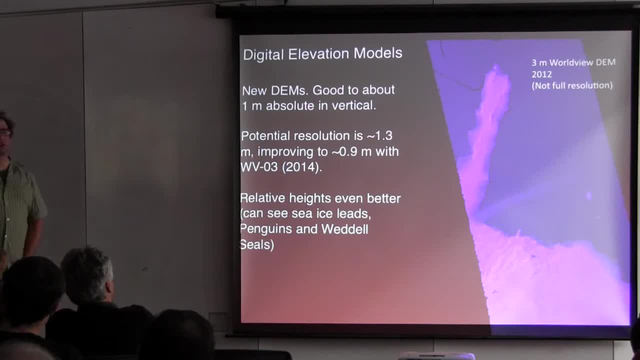 so it's about 82 centimeter resolution digital elevation models Just now. this is from effectively half-meter imagery. They're going to add quarter-meter imagery in this case. We can do relative heights very, very well If we can correct them. 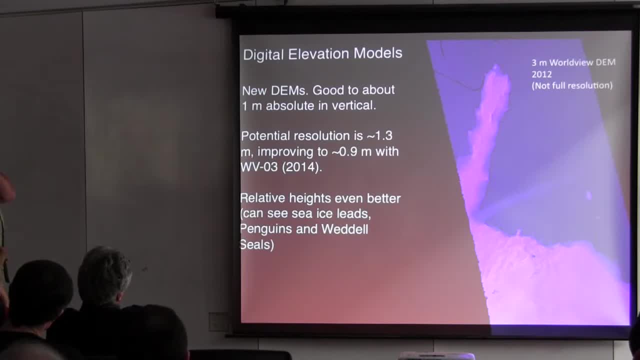 we can do absolute heights very well. You can see things like cracks in sea ice. You can see things like penguins standing around. You can see things like what else is? That's not. you can see the actual animal in the imagery. 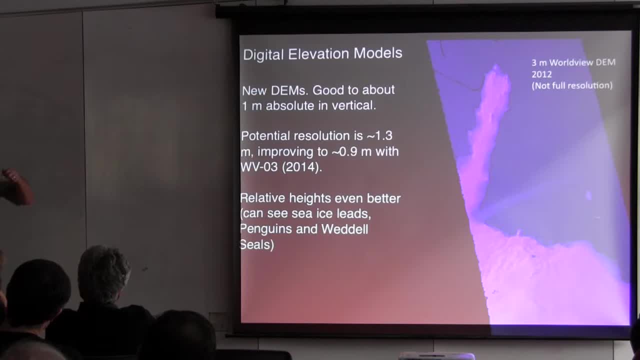 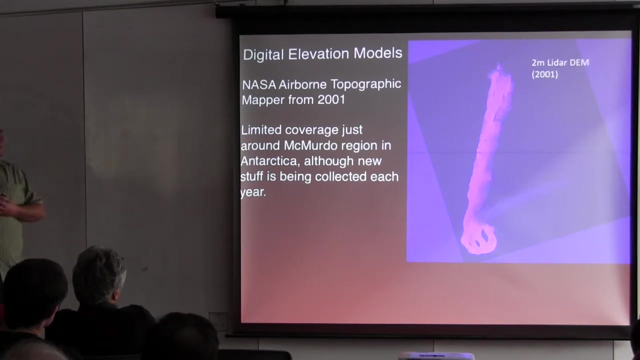 This is, we can create a digital elevation model of a seal or polar bear or a caribou sitting around on the ice with this stuff. So this is not full resolution. This is the two-meter version of the stuff that NASA flew for several million dollars. 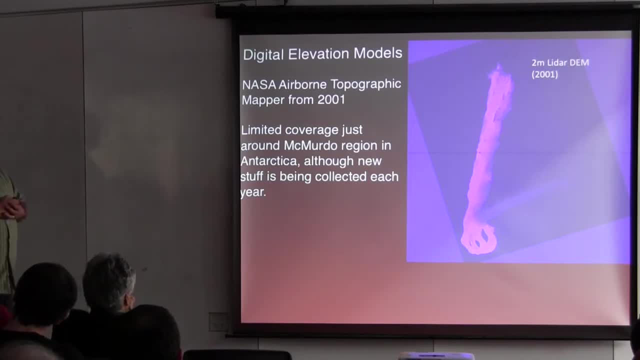 down in Antarctica in 2001.. They only did little postage stamps. everywhere The spy agencies have said: well, we're no longer tracking Osama Bin Laden, so go for it, We'll take shots of everything you want in the Arctic. So they're blasting it. 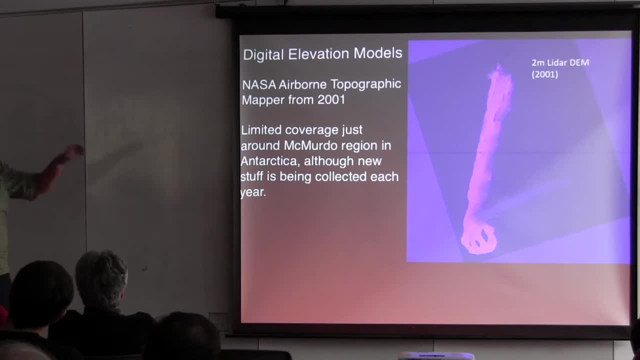 I get an email from them each weekend saying: well, we collected 450 images for you this week, or 200 images last week. So I then get to go and load up my new computer. I spent $13,500 on hard drives a couple of weeks ago. 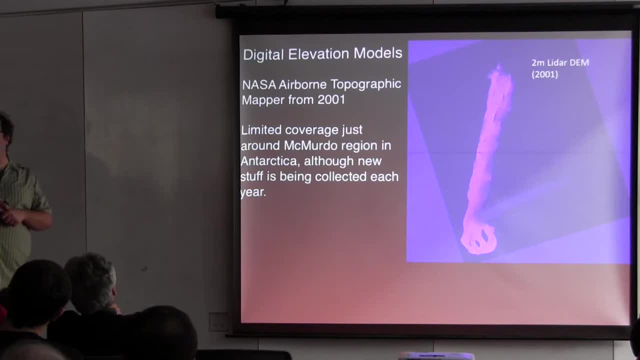 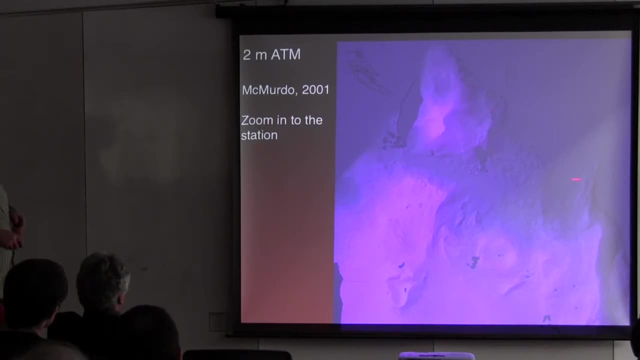 Because these things are big. What kind of a car is that? This is what the laser altimeter says. McMurdo, looks like you've got fuel storage tanks here. This is the. this is the main science building. Here's the. 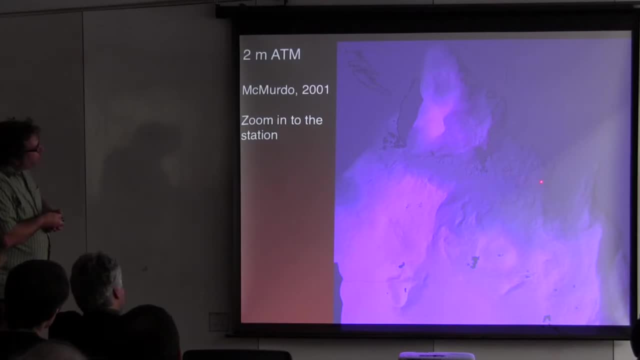 actually there's the main science building, Here's the galley. You've got the. they call them the college dorms and it's sometimes like that, Down here, a crater at the top of the hill, The different roads coming out of it. 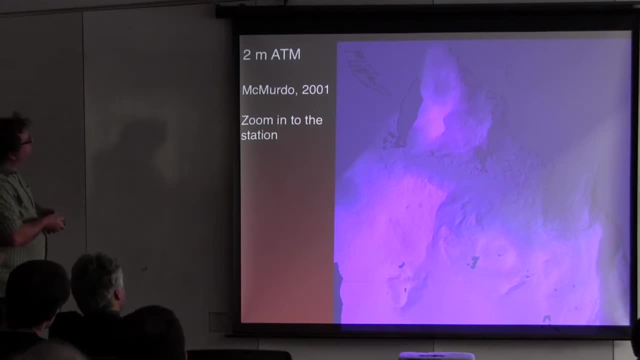 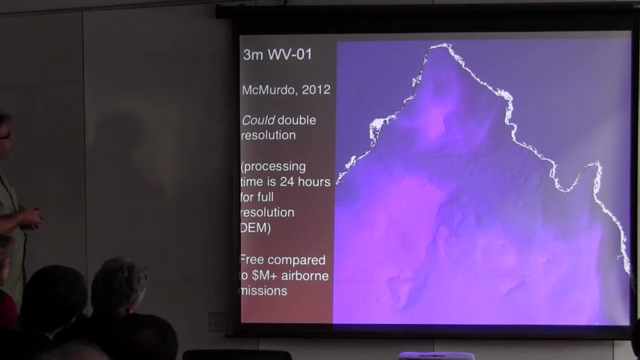 They have some wind generators up here Now, so that's two meters that you got from, I said, a couple million dollars worth of input to get that. This is the three meters that could go two meter and a half from 770 kilometers away for free. 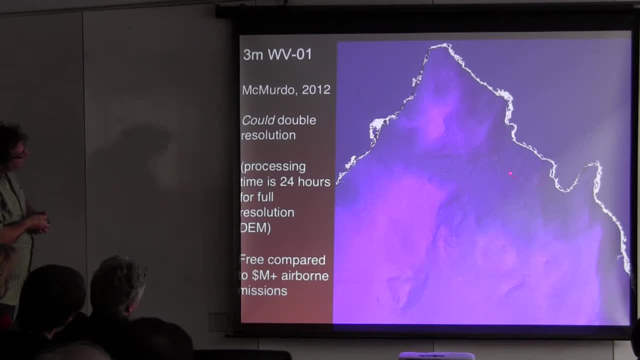 So I'll take it for free. Thank you very much. Again. we can kind of see the buildings. They're a bit spewed out. We can see the fuel tanks there And we've got this from 2012.. There's the crater again. 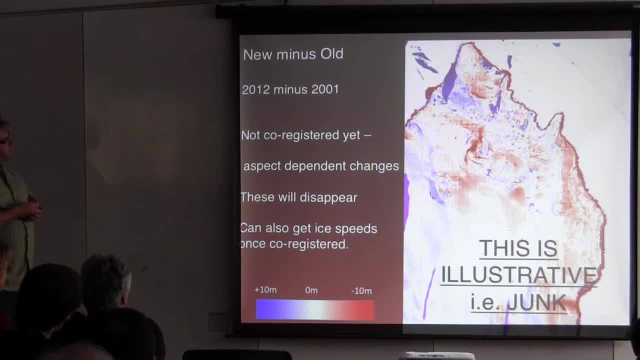 And then you can take the new one minus the old one, And oh, there's your fuel tanks, There's your buildings. Now, this isn't wonderful. What's happening here is the two DEMs are slightly offset. So once we correct that, 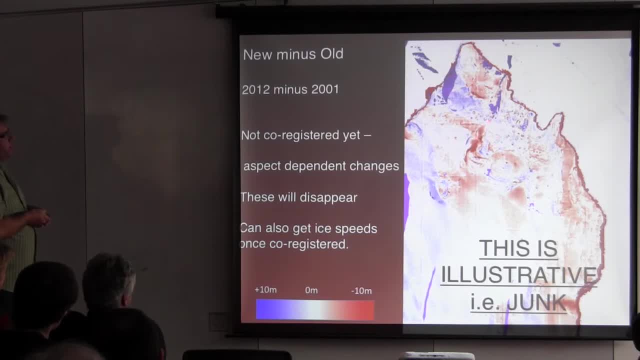 a lot of these will disappear, Although some of them might. if a fuel tank has been built, we'll be able to tell you the volume of the fuel tank, Because it wasn't there in one image. It is there in the second image. 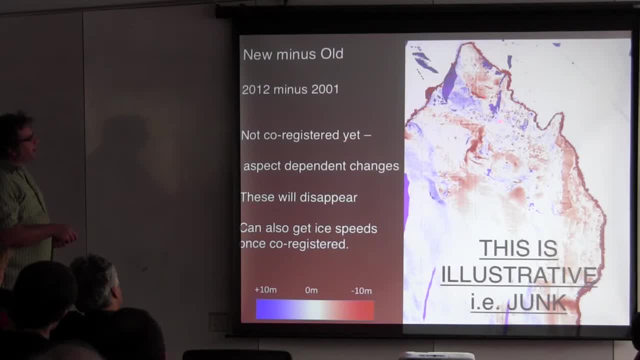 But once we co-register this, these aspects dependent changes will disappear. So basically, this is illustrative. It's junk, but it kind of tells you where we're going And we plan on doing this, for this won't take forever. 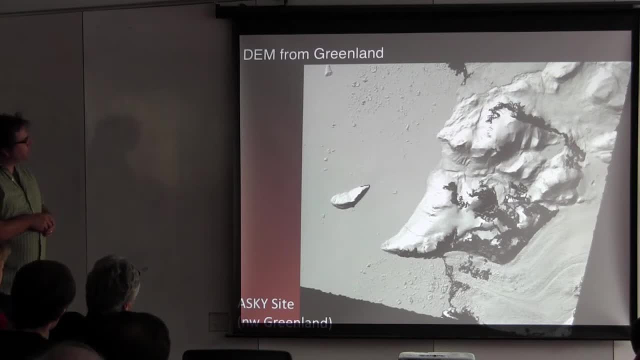 So this is a Greenland glacier- about three meters as well, And you can see the glacier coming down here and all the icebergs coming off the front of the glacier. This isn't a picture, This is a topography. So this is heights. 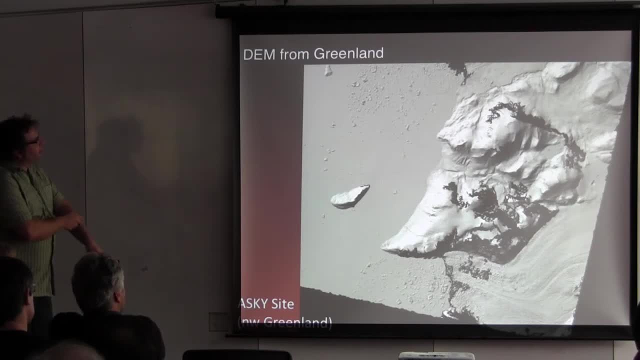 So it's spectacularly accurate, And we get into problems when, if we do a difference with this and the glacier has moved a bit, what was a crevasse is now a ridge between a crevasse, And so we have to sort out. 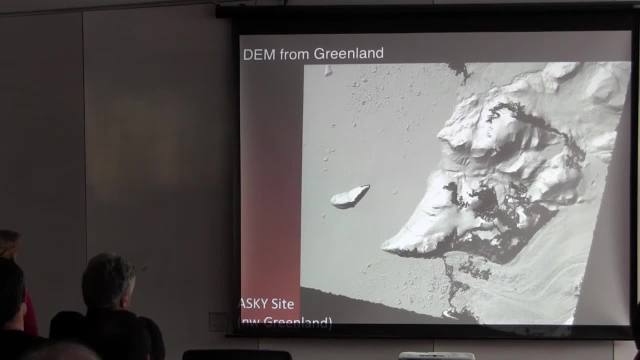 is this actual thinning or is it just a crevasse? It's a crevasse moving through our imagery, But I've started building these for Greenland. We have lots of these for the Russian Arctic. We have potential to get them for Patagonia. 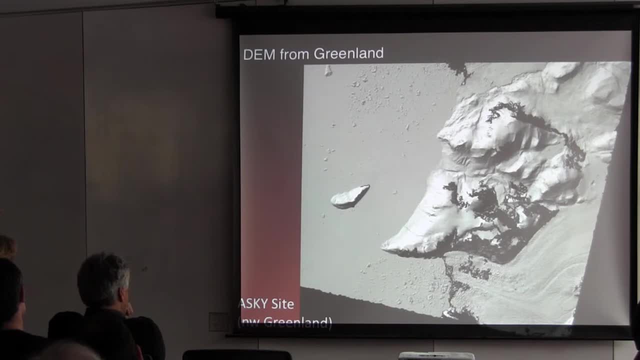 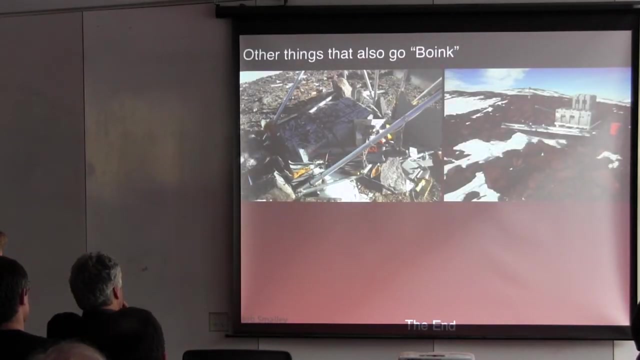 We're getting them for Antarctica, We've tasked them to do stuff for Alaska, So hopefully we'll just be getting more and more and more of these in a production mode so we can start doing these elastic corrections, Some other things. This is the last slide.